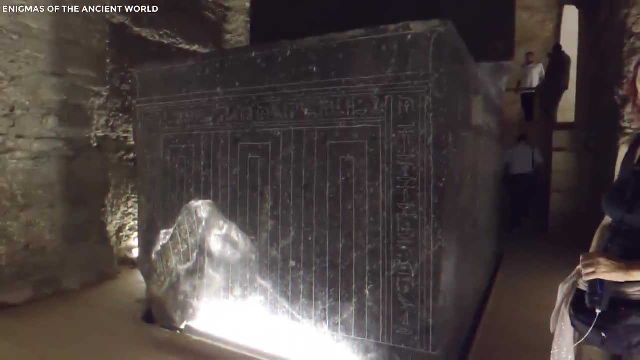 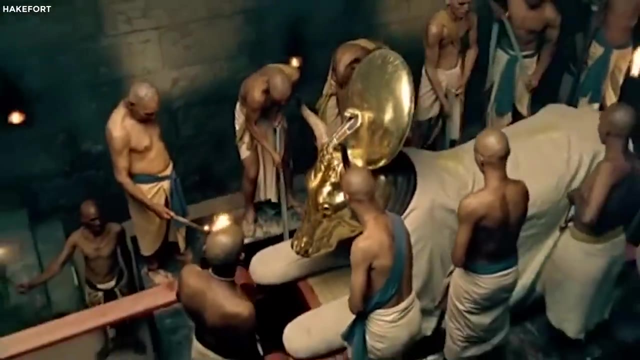 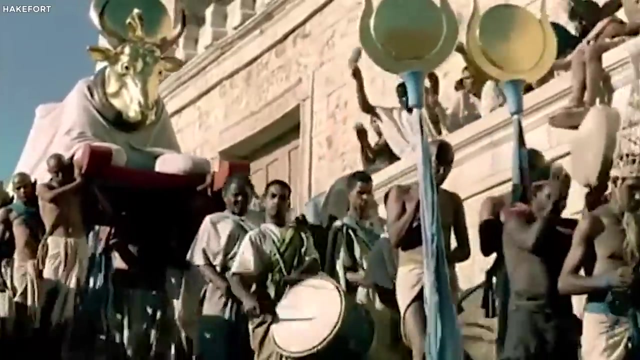 The mystery surrounding the Serapium doesn't end there. Despite being excavated for over a century, researchers are still trying to piece together why these sacred bulls were given such a grand burial. Some believe they were seen as physical manifestations of the god Apis, while others believe they were symbols of fertility and renewal. It's like a juicy. 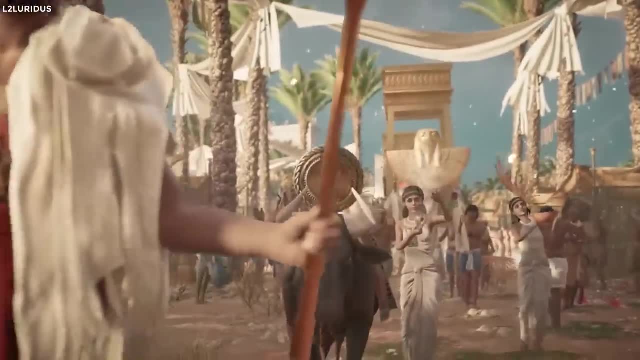 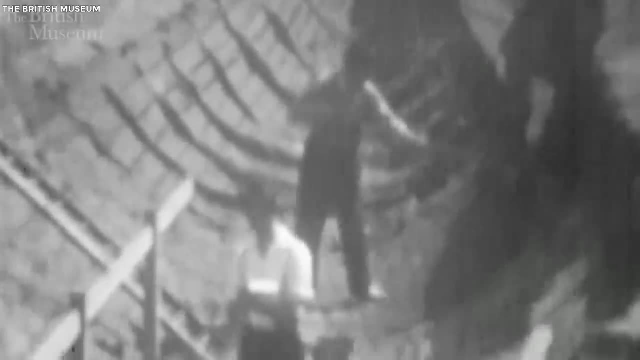 conspiracy theory. only this time the conspiracy involves sacred cows. 19. Sutton Hoo. Let us move forward to Sutton Hoo, the most glamorous archaeological site in all of England. Picture this: It's the year 1939, and a woman. 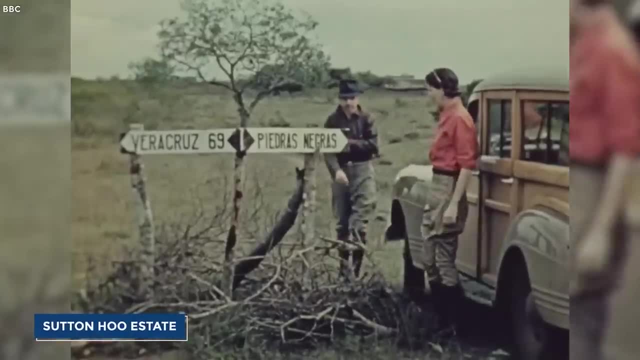 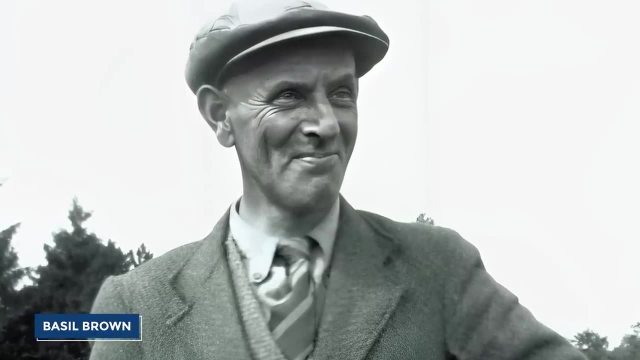 named Edith Pretty has just purchased the Sutton Hoo estate. Little did she know she'd hit the jackpot One day. she hires a local archaeologist named Basil Brown to come and do a little digging And then, BAM, He hits something hard. It's not a rock, it's not. 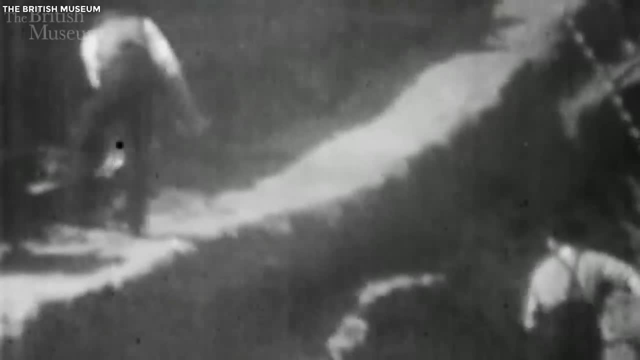 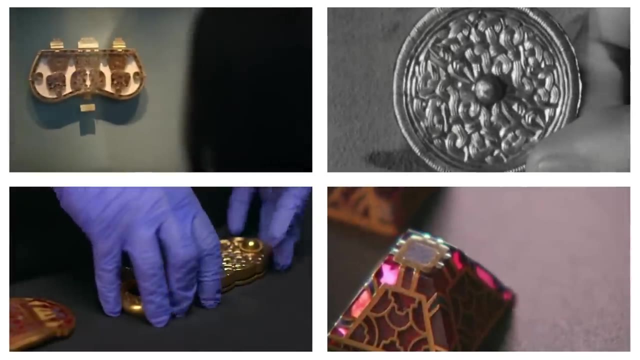 a root. it's a ship burial. That's right, a ship burial. So they start digging And they find this huge ship buried under the earth. And they find it buried under the earth And inside the ship is a treasure trove fit for a king, Literally, They found the remains of a king. 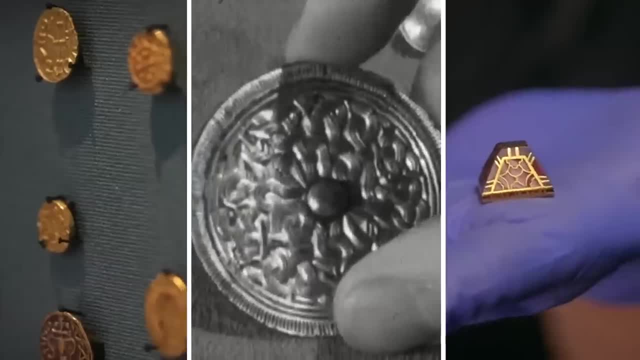 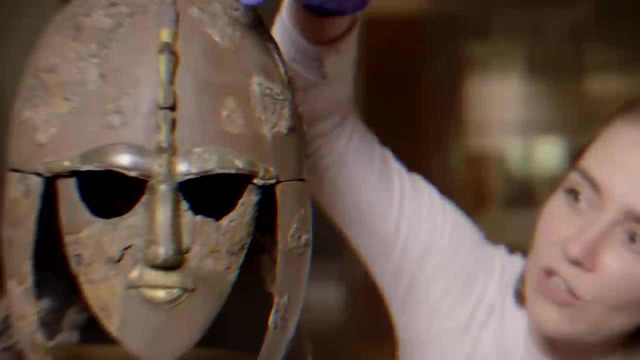 along with all of his bling bling. There were gold coins, silver dishes, precious stones, you name it. It was like the Anglo-Saxon version of Tiffany's jewelry box. They found a helmet that was so fancy it would make Lady Gaga jealous. It had gold garnets and a face mask. Yes, 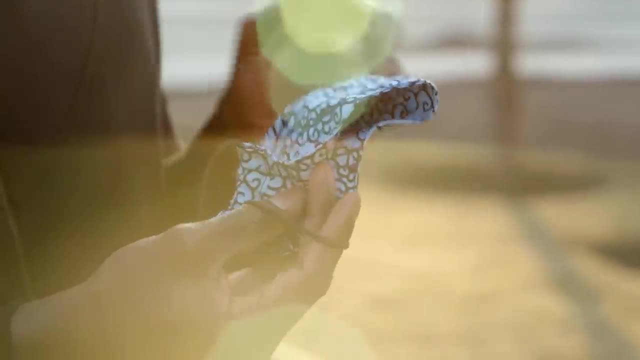 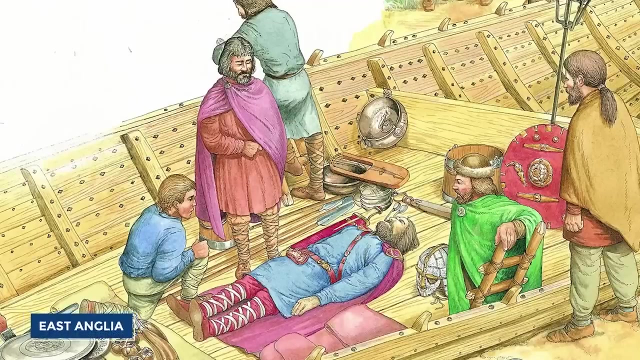 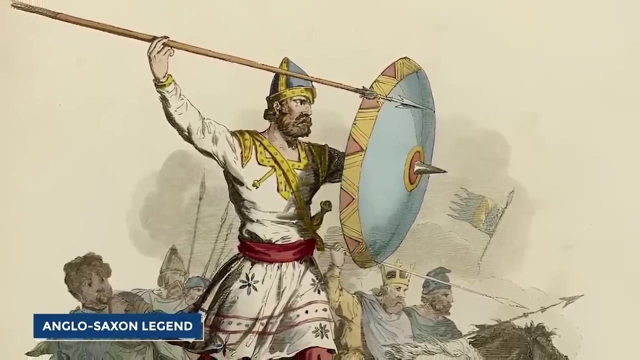 a face mask. And we thought face masks were a new thing. Historians strongly suspect that Sutton Hoo was the resting place of the Woofingas, the royal dynasty of East Anglia. They claim descent from Woden himself and their story is woven into the fabric of Anglo-Saxon legend. 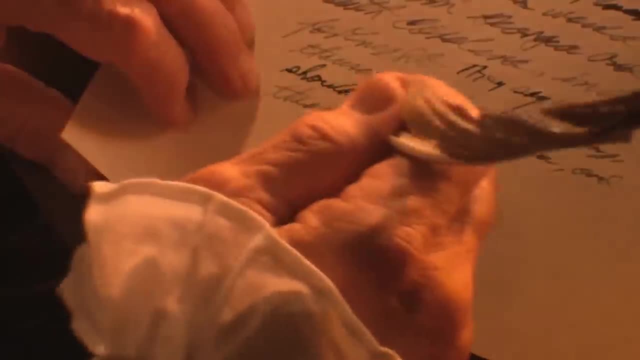 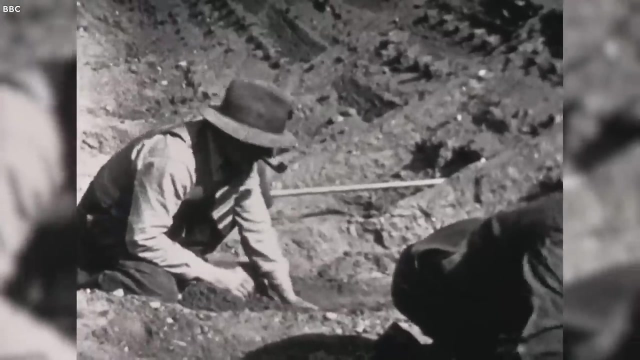 Imagine that, tracing your lineage all the way back to a god, But sadly there are no written records to tell us their story. Sutton Hoo, where the treasure is as fabulous as a drag queen and the curse is as real as a Kardashian wedding. 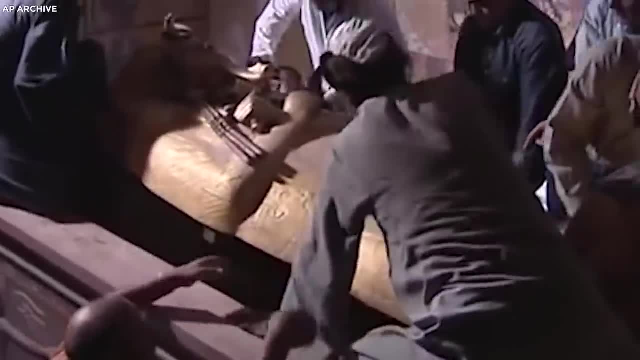 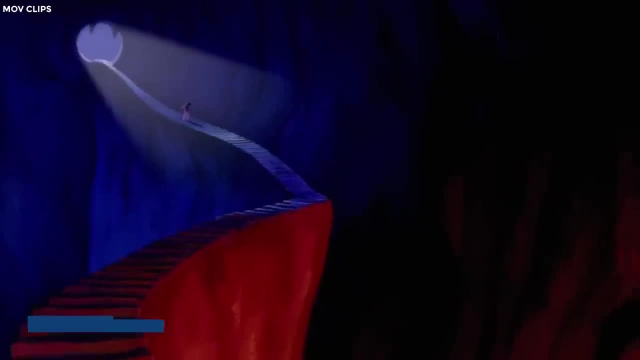 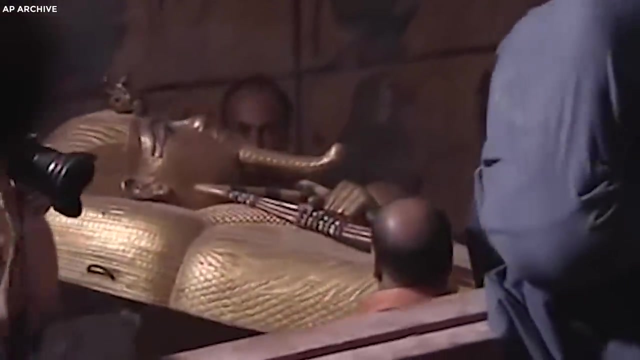 Now we have the most epic tomb of all time, the one and only King Tutankhamun's resting place. First off, do you remember the scene from the movie Aladdin where he discovers the Cave of Wonders? Well, imagine that, but on steroids: From golden sarcophagi to dazzling jewelry. 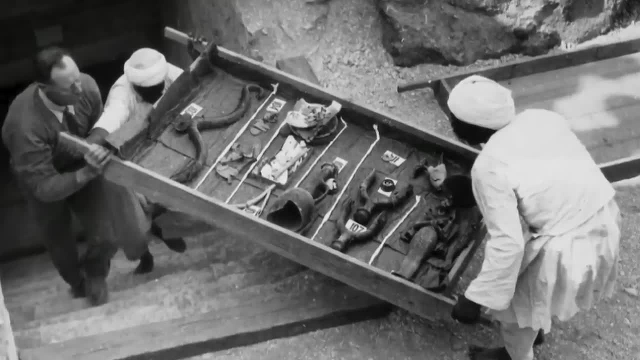 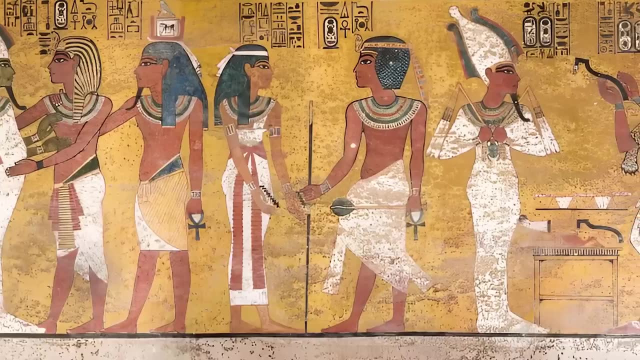 King Tut's tomb is like a treasure hunter's dream come true. As we wander through the winding corridors, we're struck by the sheer opulence of it all. There are priceless artifacts, intricate carvings and detailed hieroglyphics adorning every inch of the walls. 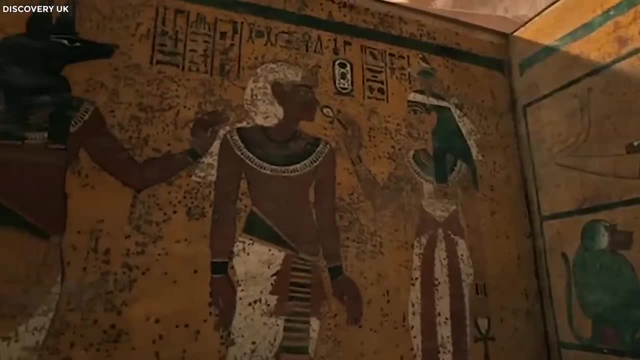 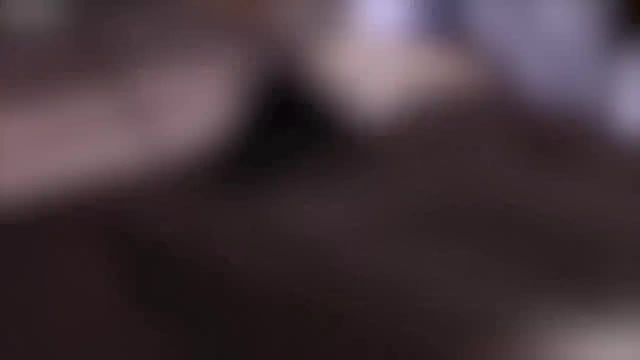 It's enough to make your head spin. And then, just when we think we've seen it all, we come to the Piste de resistance, the burial chamber of King Tutankhamun himself. You almost expect the King himself to rise from his slumber and greet us, But we are better off without it. 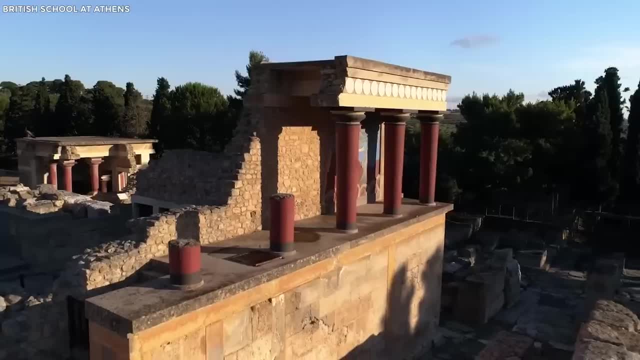 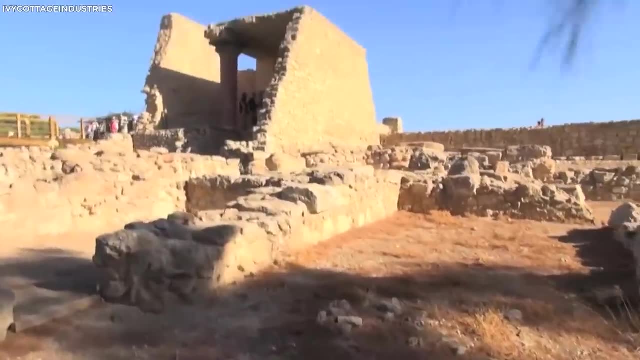 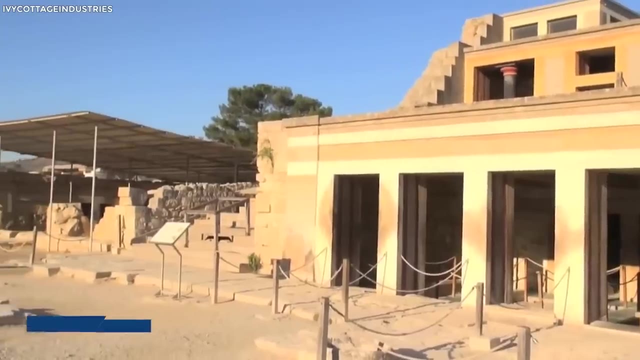 17. Knossos. Let us move forward to Knossos, the ancient version of Disneyland. except instead of Mickey Mouse, you've got minotaurs and mystical ruins. Nassos, the city that time forgot, was the center of the Minoan civilization that thrived on the island. 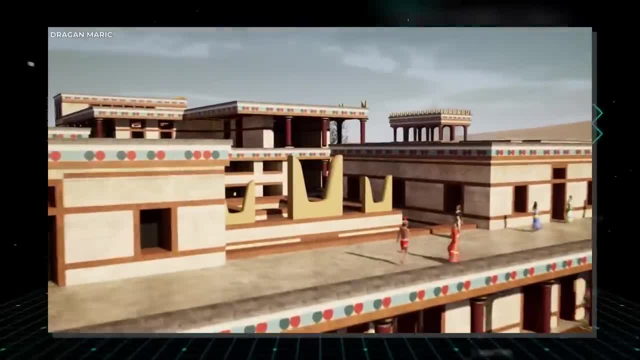 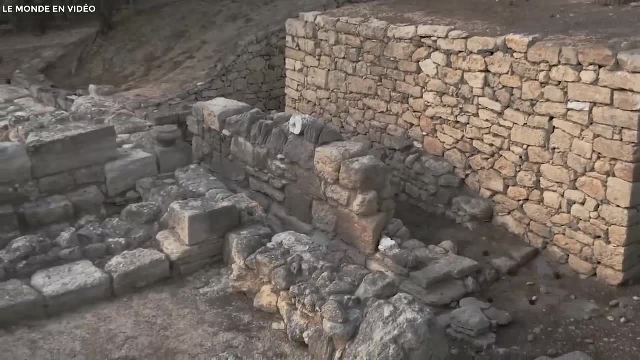 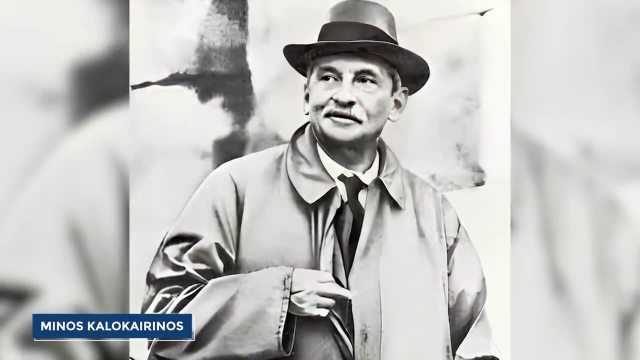 of Crete during the Bronze Age. It's like the OG of ancient cities with a history that dates back to 7,000 BC. And let's not forget the epic archaeological discovery that took place in 1878, when the amateur archaeologist Minos Kalokairinos stumbled upon the palace complex of Gnosos. 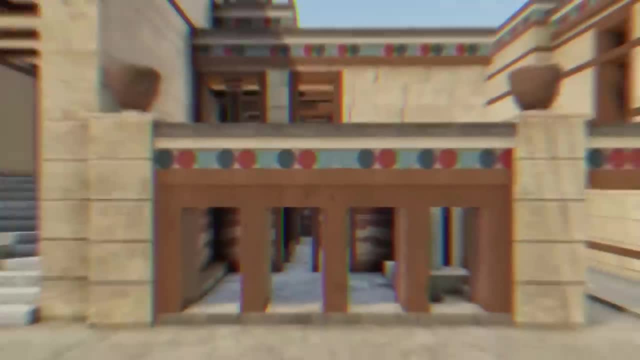 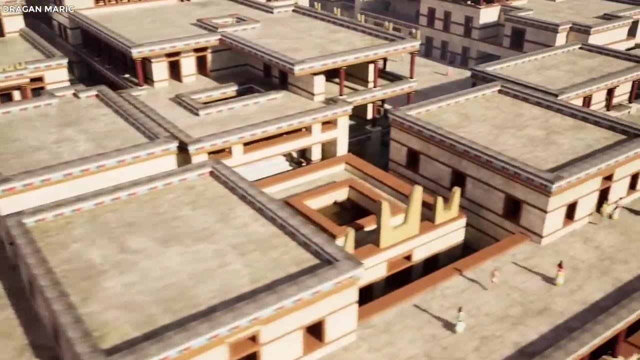 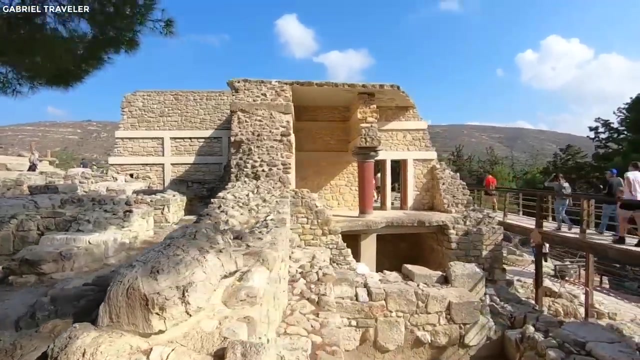 And then there's the palace complex itself, with its 1,300 intricately decorated rooms that probably housed the most powerful and wealthy people of the time. And then there are those baked clay slabs with inscriptions still unknown, almost as if they're taunting us. 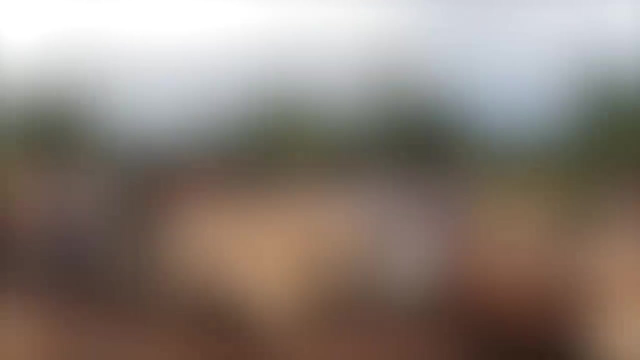 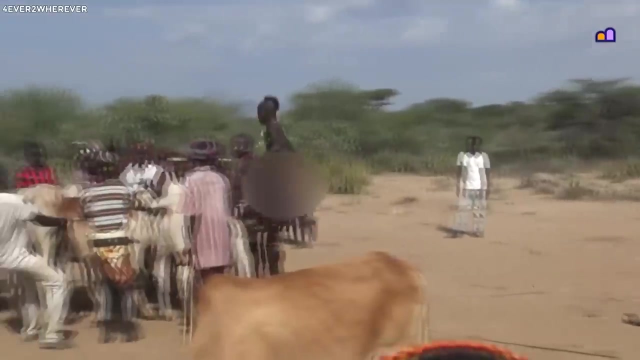 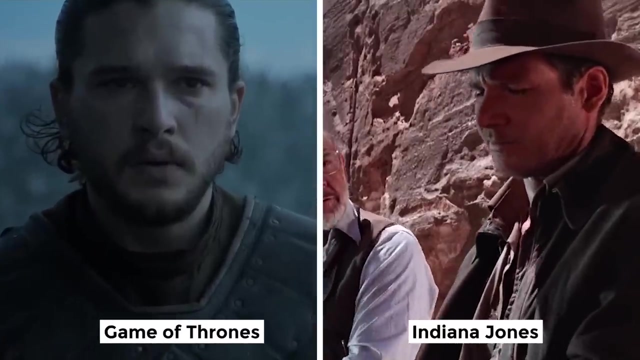 daring us to try and decode their secrets. But the real kicker is that the palace complex itself is a place where the people of Crete is the bull jumping ceremony. It was an original extreme sport, a ritual where young men and women would vault over a bull's back in a display of strength and courage. It's like if Game of Thrones. 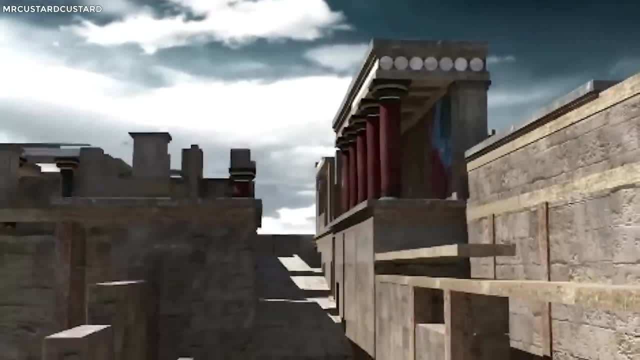 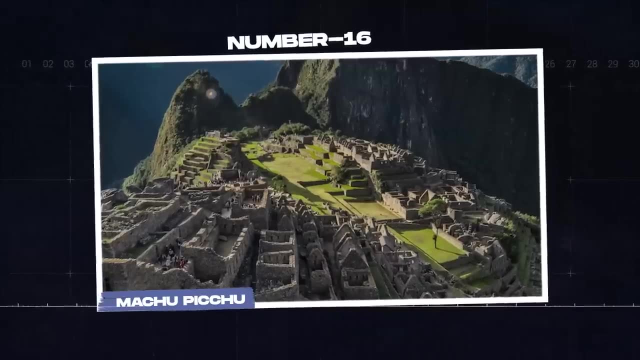 and Indiana Jones had a love child, and that love child was an ancient palace complex on the island of Crete. 16. Machu Picchu: Now hold on to your llamas, because we're about to embark on a journey to the legendary Machu Picchu. 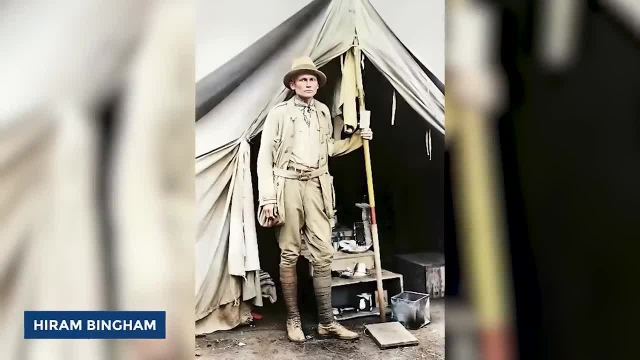 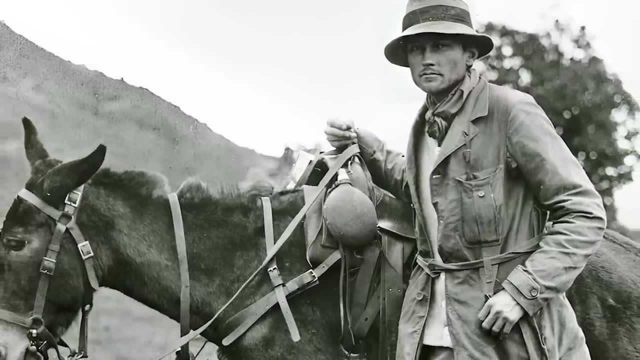 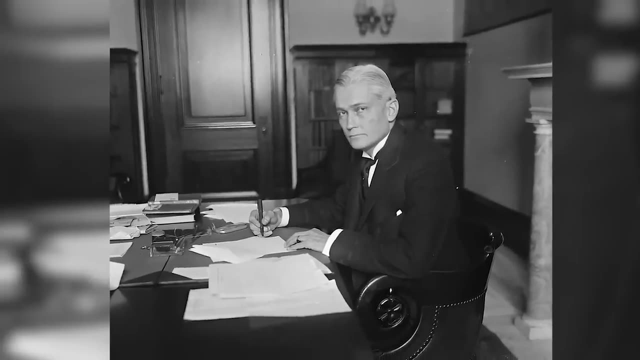 the mystical land of the Incas. Let's talk about Hiram Bingham, the man who rediscovered Machu Picchu in 1911. He must have been channeling his inner Lara Croft, because he stumbled upon this lost city like it was nobody's business. And boy are we grateful for his discovery, because this place 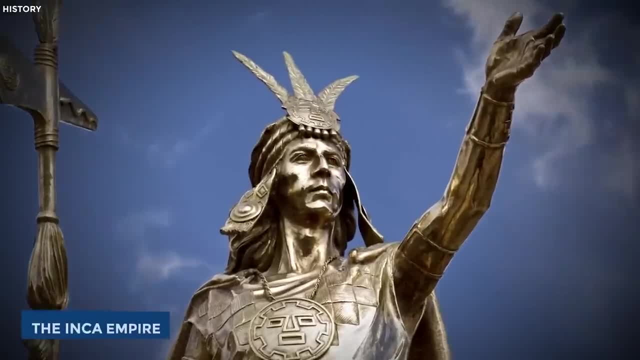 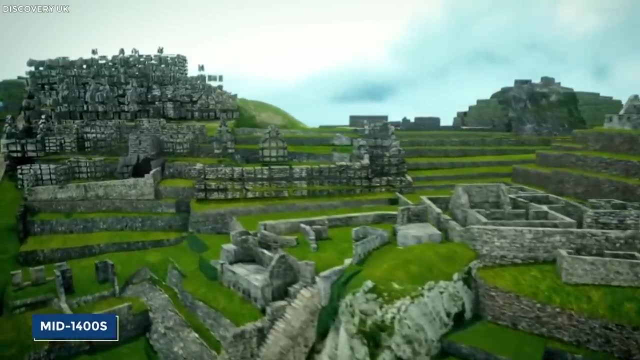 is a total showstopper. On to the basics, The Inca Empire, at the peak of its power, constructed Machu Picchu during the mid-1400s. This city was constructed by the Inca Empire and it was built by the Inca Empire. 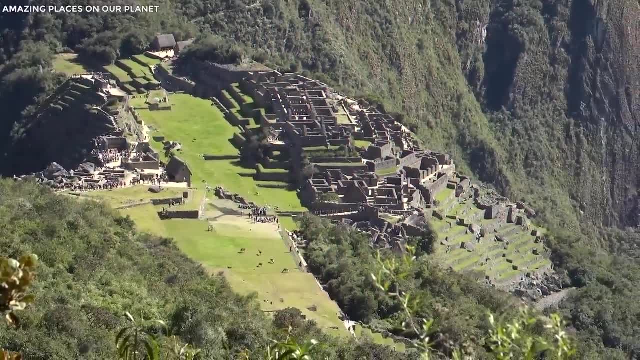 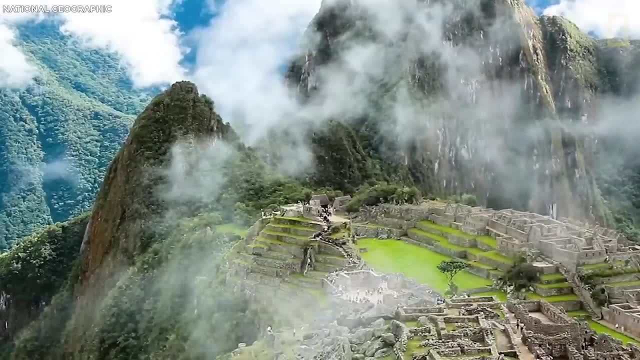 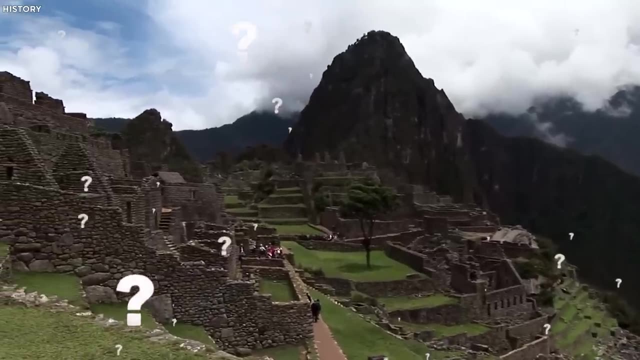 It was constructed on top of a mountain and is known for its impressive engineering feats, such as its terraced platforms and intricate water management system. But what's truly fascinating about Machu Picchu is the mystery that surrounds it. For example, there is the question of the purpose of the city. 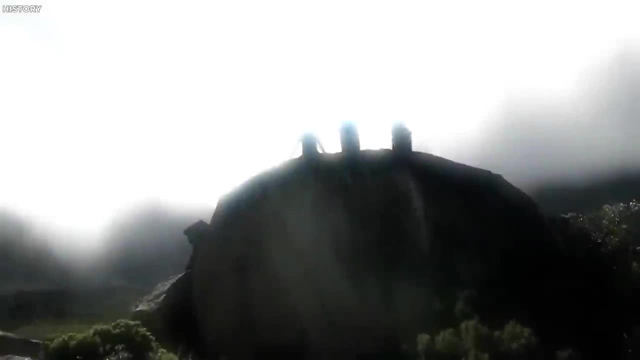 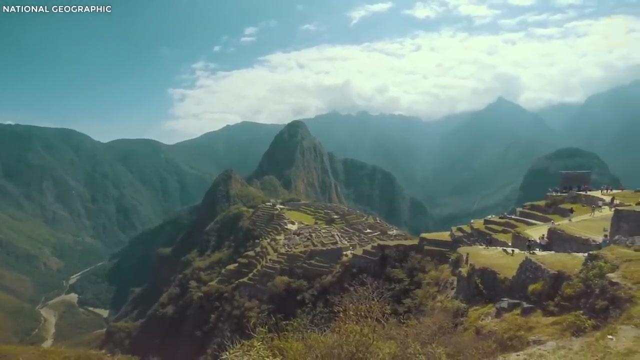 Was it a military base? Was it for royalty? Was it for the sake of religion? Too many possibilities and never-ending curiosity. And don't even get started on the panoramic views from the top of Machu Picchu. It's like a postcard come to life. 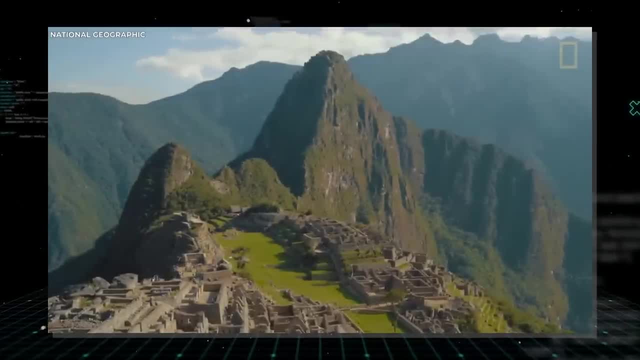 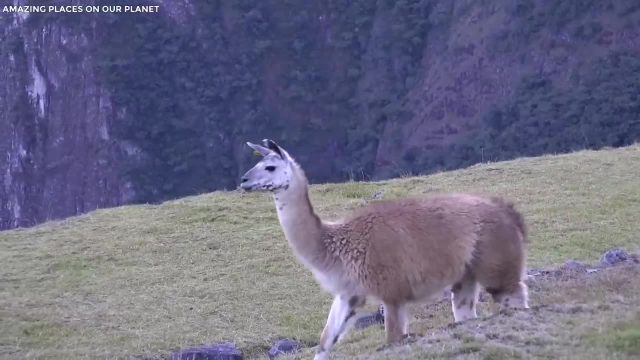 with lush greenery, cascading waterfalls and endless mountain ranges as far as the eye can see. And let's not forget about the llamas. These fluffy four-legged creatures roam the city like they own the place. It's no wonder this place has been declared one of the 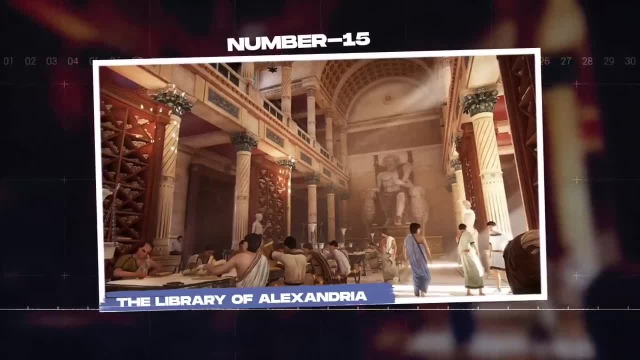 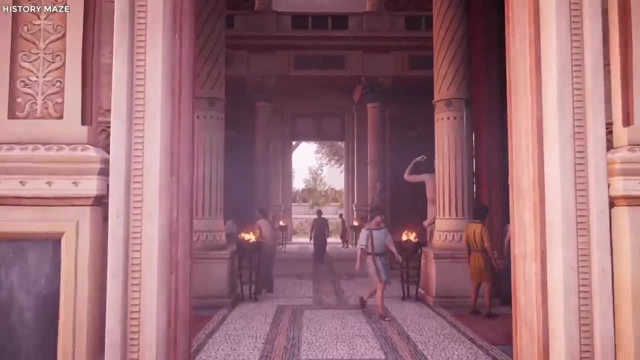 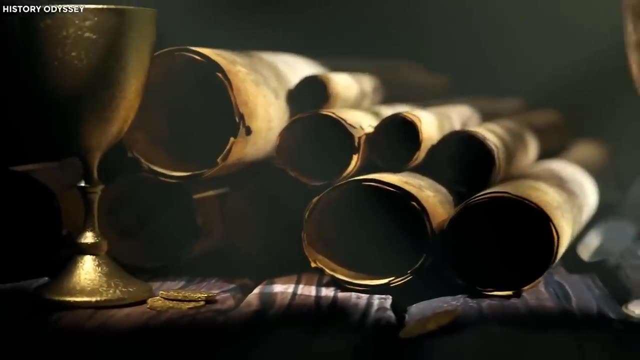 seven wonders of the world. 15. The Library of Alexandria. The Library of Alexandria, our next stop, is one of the most legendary libraries in history. It is like Hogwarts of the ancient world, but instead of finding magic spells, there are scrolls And honestly, those scrolls and books. 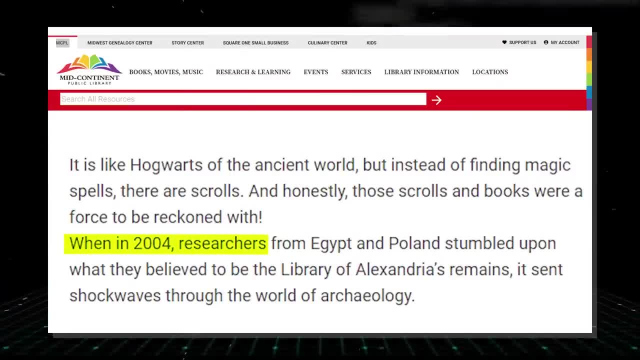 were a force to be reckoned with. When, in 2004,, researchers from Egypt and Poland stumbled upon what they believed to be the Library of Alexandria's remains, it sent shockwaves through the world of archaeology Because, you see, the Library of Alexandria was not just another. 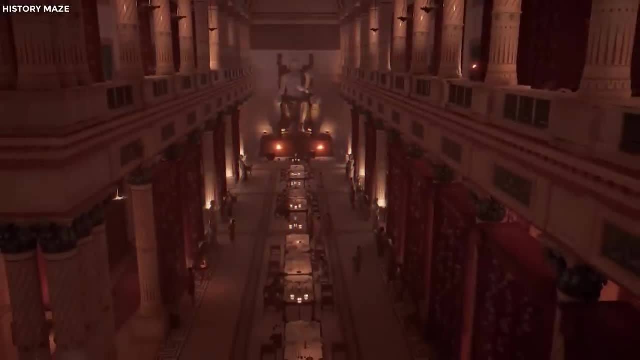 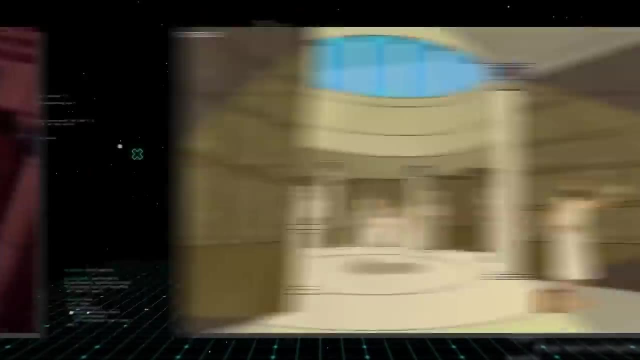 aesthetic place with mahogany shelves. It was the symbol of knowledge of the ancient world, Just like that. people did not only go there to hide in a corner and drown in a book, although that was one of their favorite activities. it was also a hub for intellectuals and scholars. 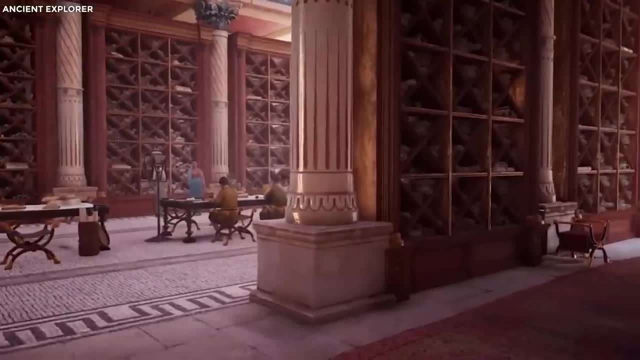 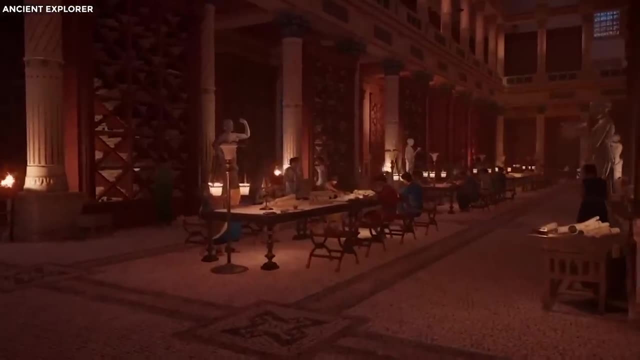 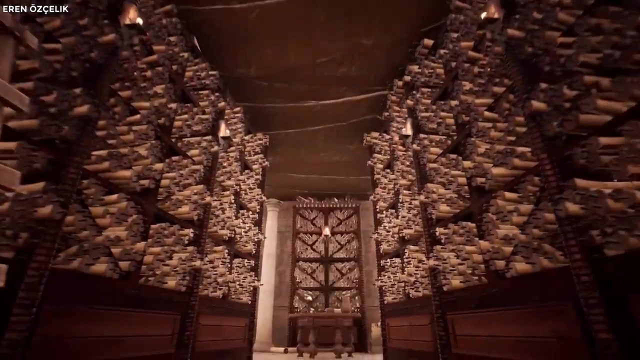 Ideas were exchanged, lectures were given and debates were held within those walls During the reign of the Ptolemaic dynasty in Egypt. they were obsessed with gathering and preserving all the knowledge of the world, So much so they would confiscate any and every book that arrived at their port. 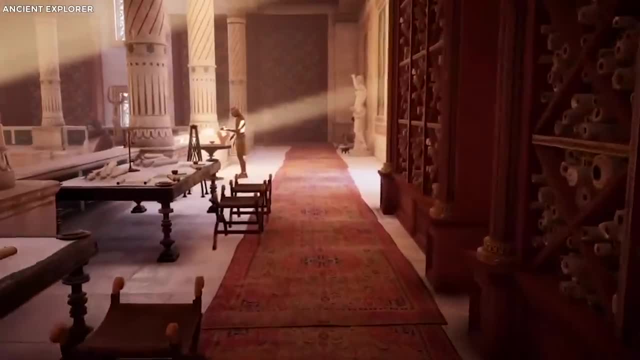 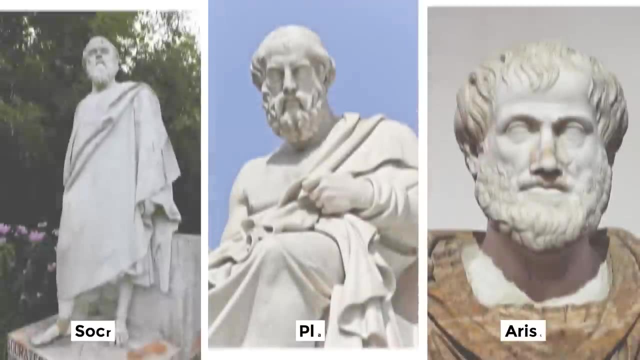 and copied it for their collection. It was a different world, where nerds were bullies as well. It is said that the library contained the jewels of ancient times as well, including Socrates, Plato and Aristotle, And, in a painful turn of events, this fairy tale of any bookworm also came to an end. The library was destroyed, and it was done by the biggest villains of all times, Humans. The blame falls on Julius Caesar by most historians, while there are speculations for a raging fire as well. Whatever the reason, it is a tragedy that still echoes through the ages. 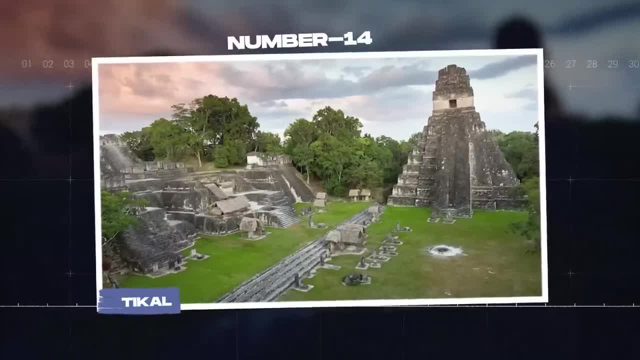 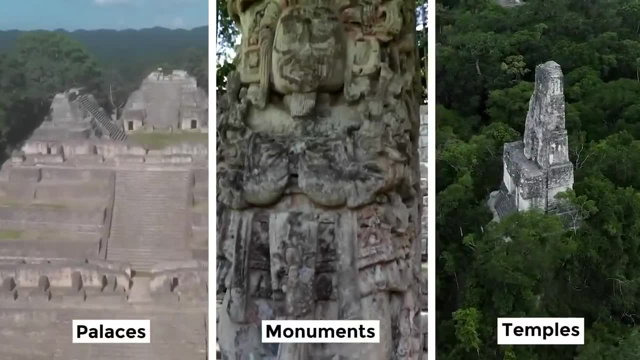 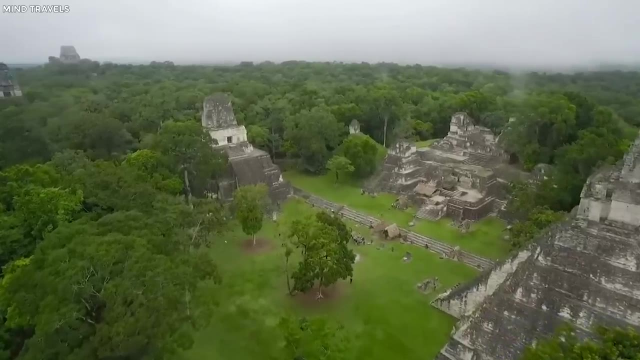 14. Tikal. Tikal is a pre-Columbian Mayan city which is like a historical theme park, with palaces, monuments and ancient temples that will leave you wanting for more. Situated in modern-day Guatemala, it was one of the most powerful cities in the Mayan world, with over 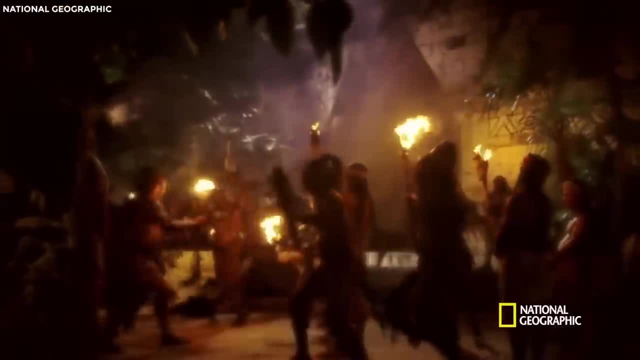 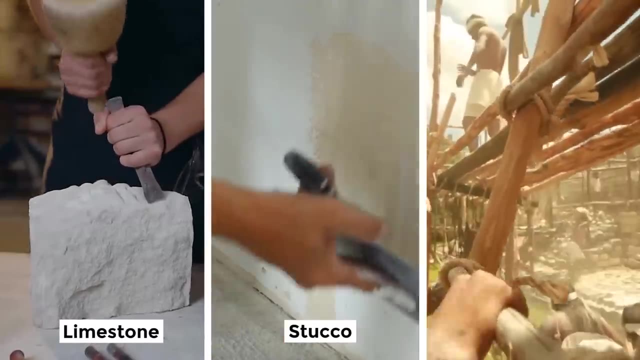 100,000 people having the time of their lives living there. As far as the eye can see, there is a range of pyramids and temples which were built using limestone, stucco and various other natural materials, Making them even more breathtaking. there are intricate 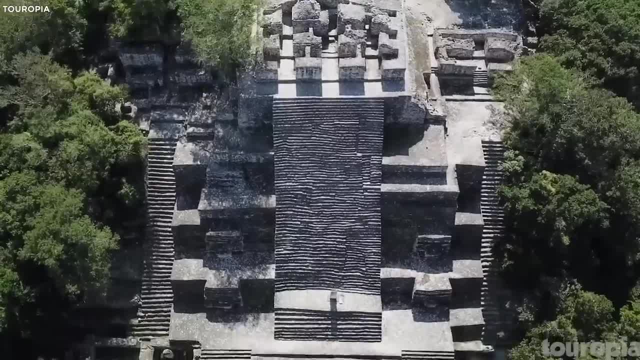 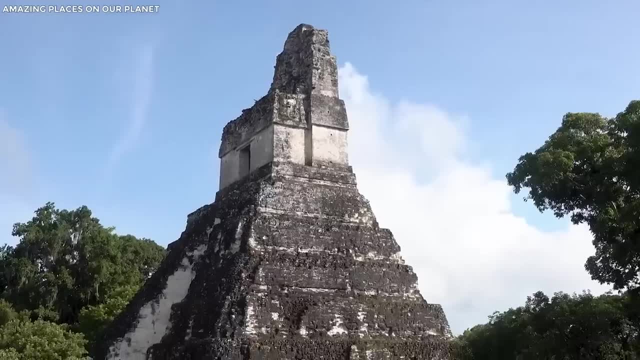 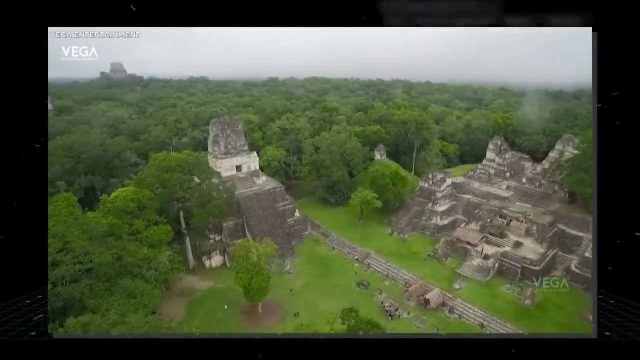 carvings and sculptures of bright colors, creating a visual effect that can give any art gallery a run for its money. But that's not all, and it only gets better. Tikal takes it up a notch with their urban design. With clever planning of the building and plazas, the city maximized space and resources for easy movement and efficient water management. 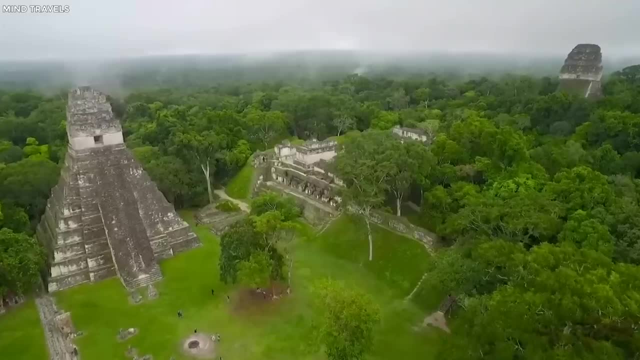 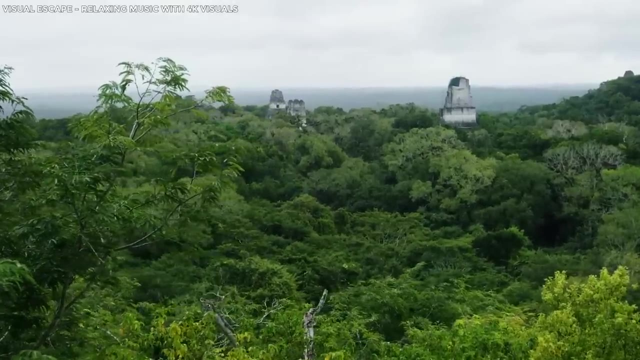 Question is: if they were so smart, why did they choose to build the city in such treacherous terrain surrounded by dense jungle? Speaking of the jungle, Tikal is a paradise for wildlife lovers. From jaguars to toucans to snakes, there is everything to intrigue and to creep. 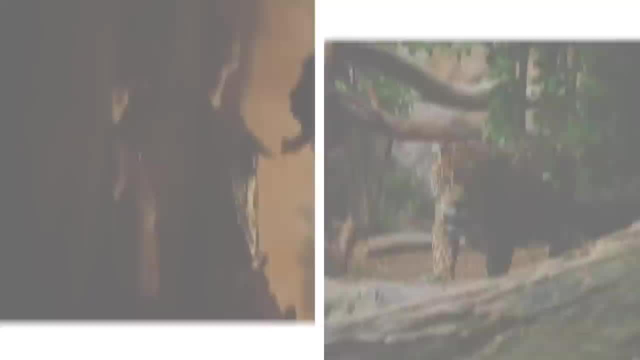 But again, what was the deal of Mayans with these creatures? Were jaguars there personally or just for fun? What was the deal of Mayans with these creatures? Were jaguars there personally or just for fun? What was the deal of Mayans with these creatures? Were jaguars there personally or just for fun? 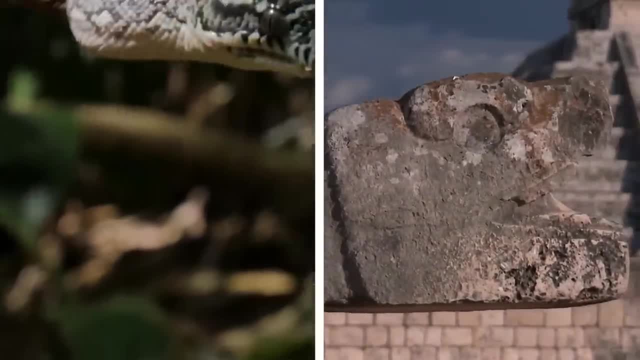 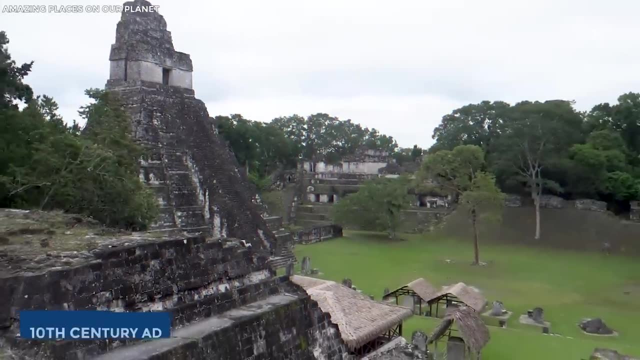 Did they have personal bodyguards or did they just hope the snakes would stay away from their sandals? Perhaps the most exciting and obviously saddening part of Tikal is its downfall In the 10th century AD. the city was abandoned and we still don't know why. 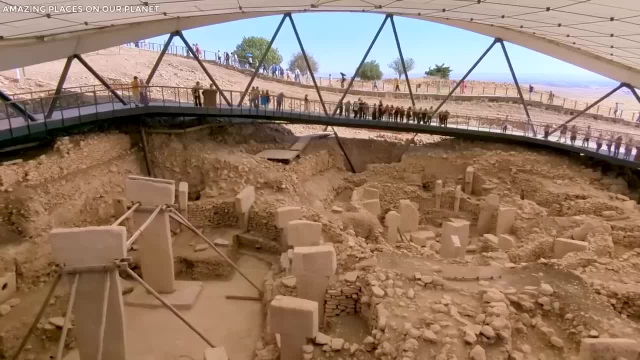 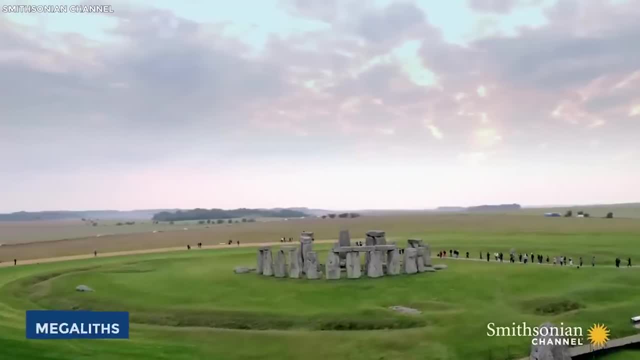 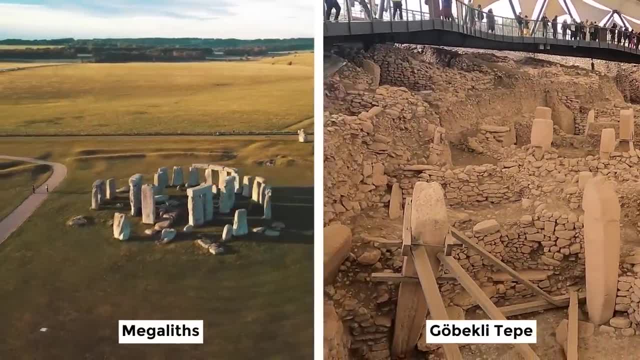 Now, if you're wondering what a megalith is, it's basically just a fancy word for a megalith, And the megaliths at Gobekli Tepe are big. Gobekli Tepe is one of the oldest known monumental architecture in the world. 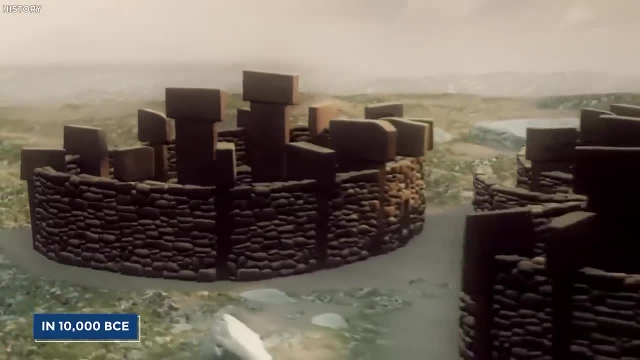 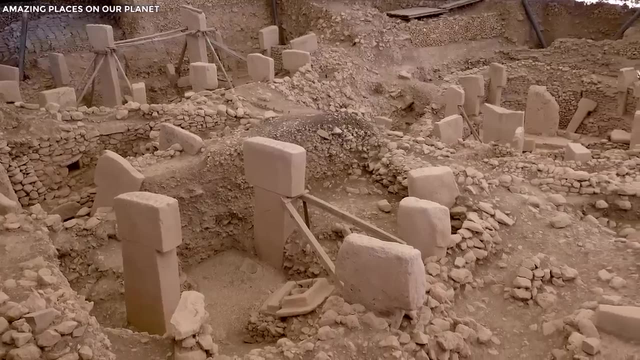 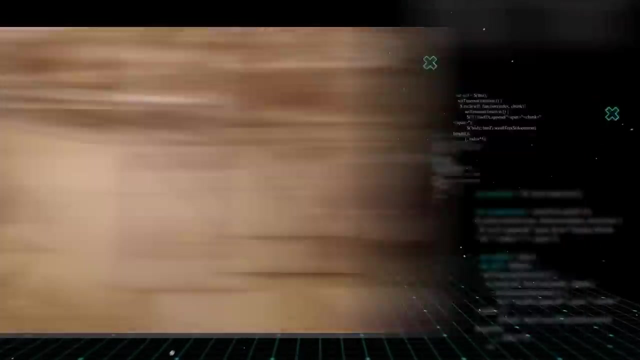 Built in 10,000 BCE. it is older than pretty much everything you can think of, even Egypt and Stonehenge, which are literally the big brothers of the ancient world. And boy, this city is like the wine of history. The carvings on the stones are so precisely done and they are arranged in such an incredible way. 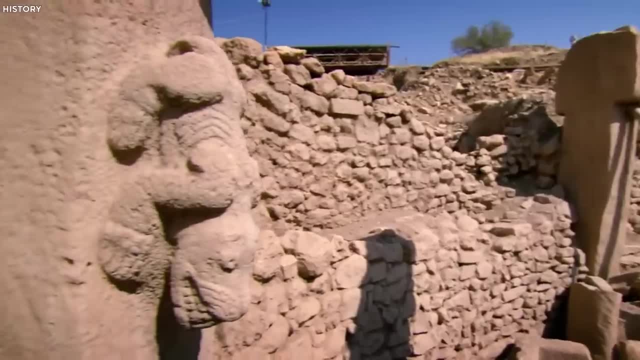 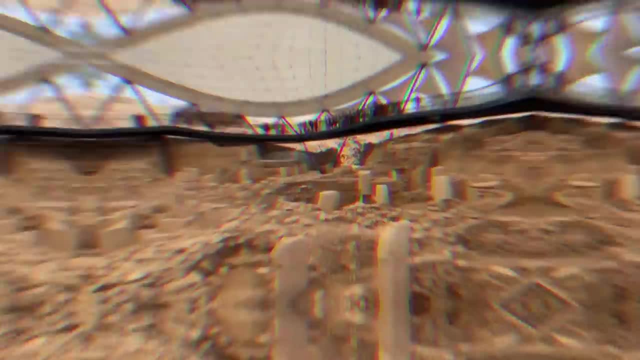 you can't help but start a fan club in their name. Honestly, they had some serious skills, and the fact that they were able to do it all without the aid of modern tools is pretty darn impressive. Can you imagine stumbling upon a site like this for the first time? 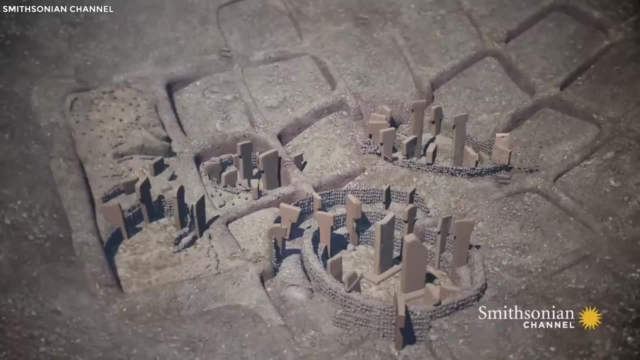 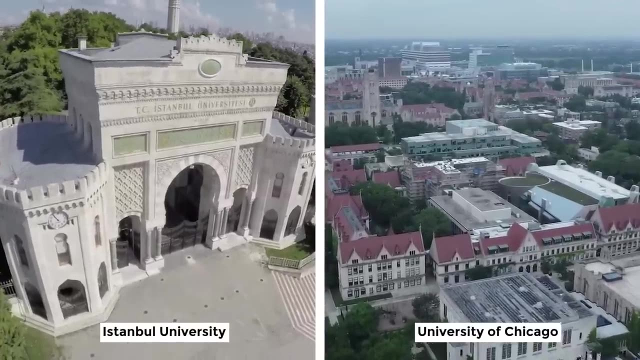 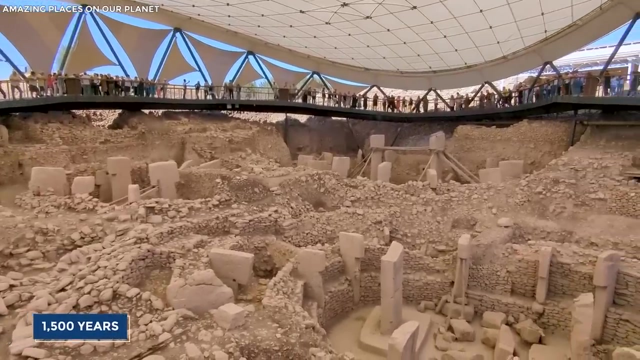 The discovery of such a remarkable historical artifact buried underground must have been exhilarating for the team of researchers from Istanbul University and the University of Chicago. And then there's the matter of why the site was eventually abandoned After around 1,500 years of use. 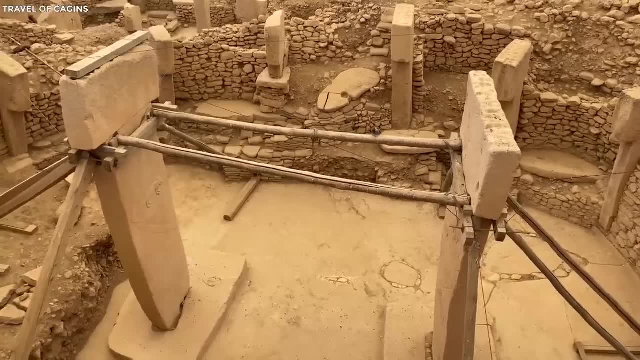 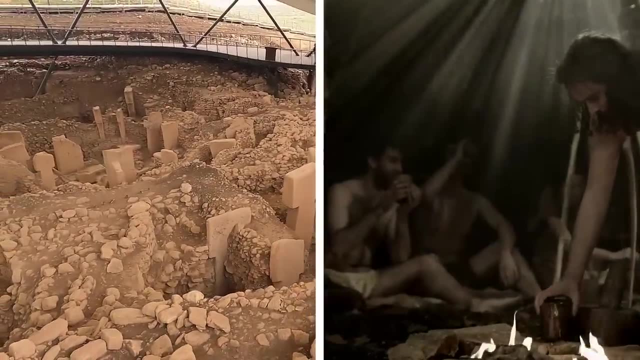 the megaliths were buried and the site was abandoned. But what we do know is that the discovery of Gobekli Tepe has forced us to rethink our assumptions about the capabilities and sophistication of our ancient ancestors. 12. Frozen Siberian Mummies. 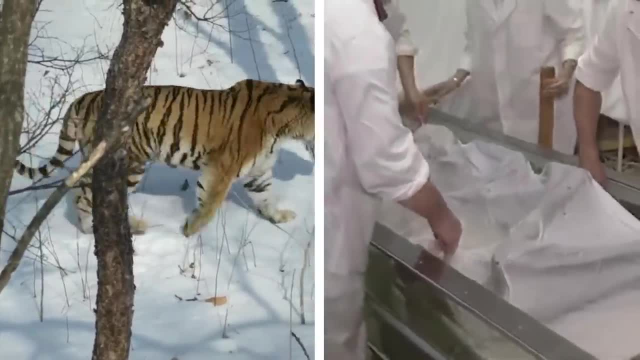 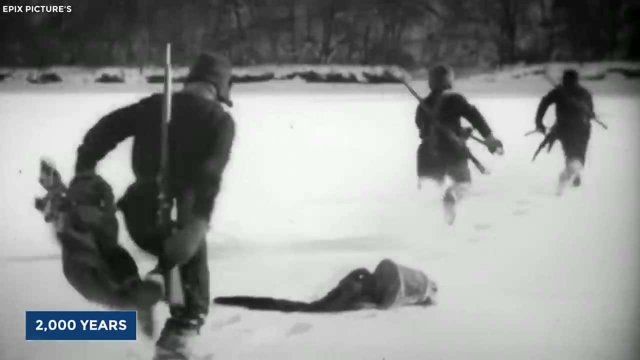 Did you know Siberia does not only have great tigers, but also has frozen mummies? They belong to a group of ancient warriors called the Scythians, who roamed the Siberian steppe over 2,000 years ago. The mummified 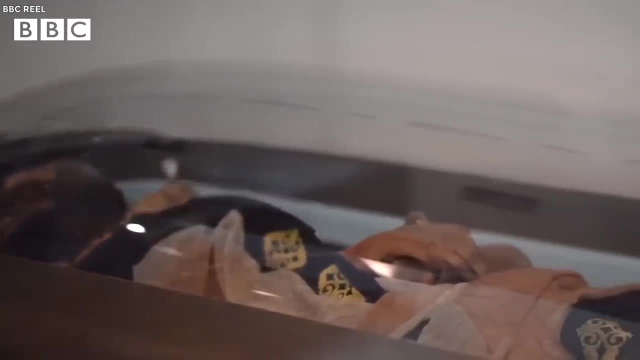 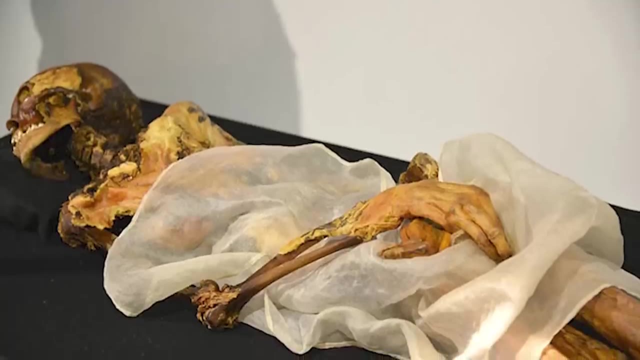 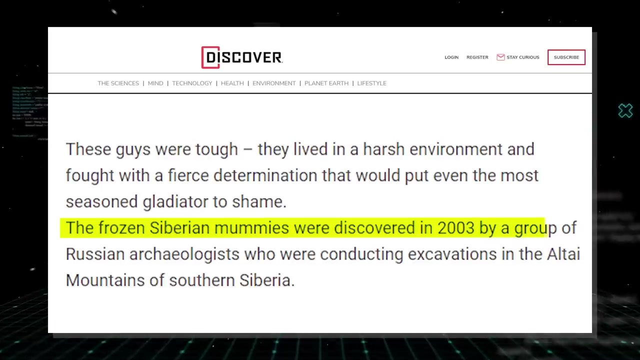 remains were so well-preserved that they appeared as if they had only recently died. These guys were tough. They lived in a harsh environment and fought with a fierce determination that would put even the most seasoned gladiator to shame. The frozen Siberian mummies were discovered in 2003 by a group of Russian archaeologists. 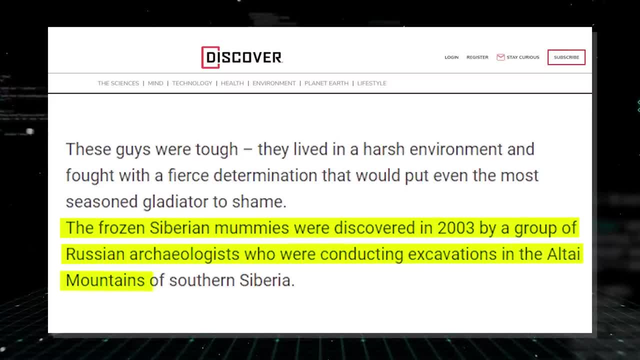 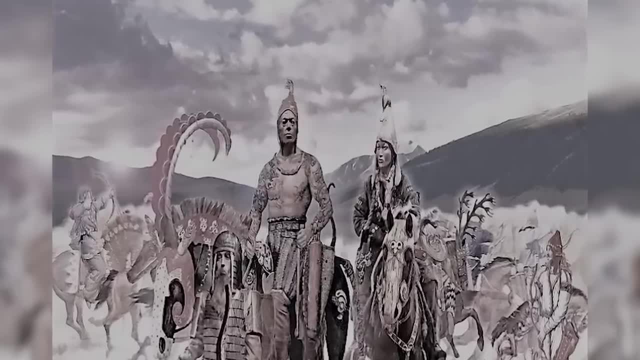 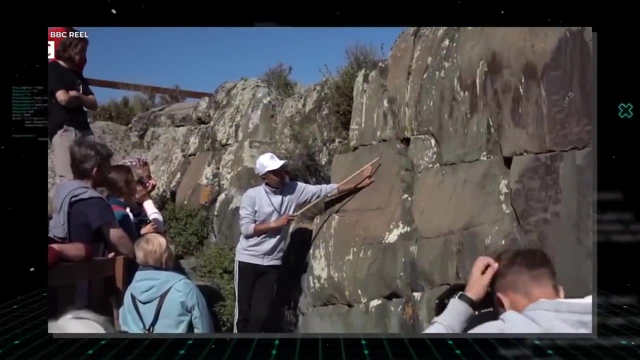 who were conducting excavations in the Altai Mountains of southern Siberia. This allowed researchers to study the remains and gain a better understanding of the Scythian way of life, including their diet, clothing and weaponry. They even found evidence of some of the earliest known battlefield surgeries. 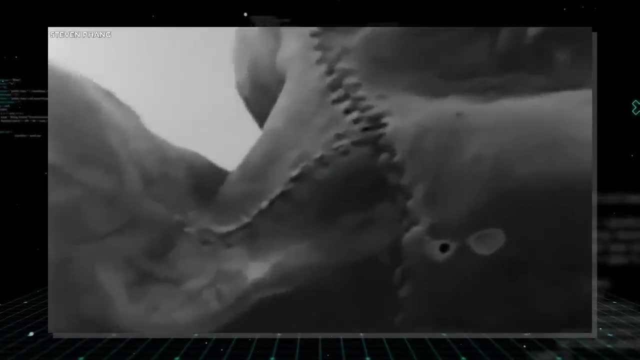 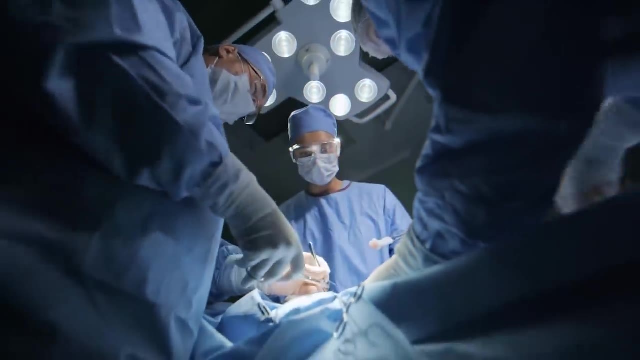 which involved tree panning or the drilling of holes in the skull to relieve pressure. Who needs a fancy hospital? when you have a sharp knife and a steady hand, You do Take your meds on time. One of the most fascinating aspects of the discovery is the presence of a slain warrior. 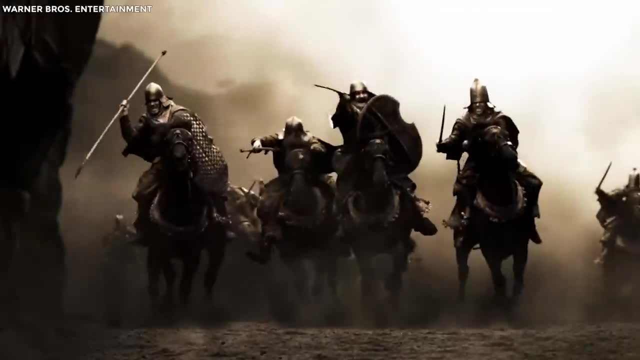 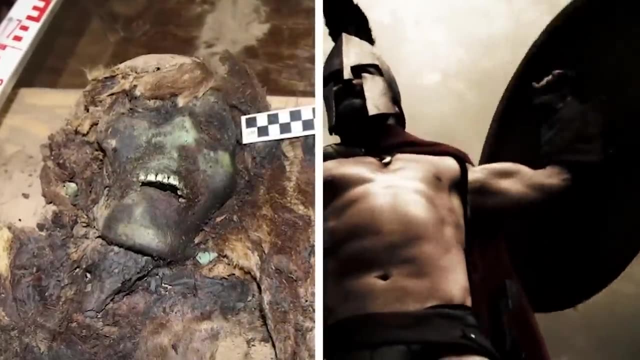 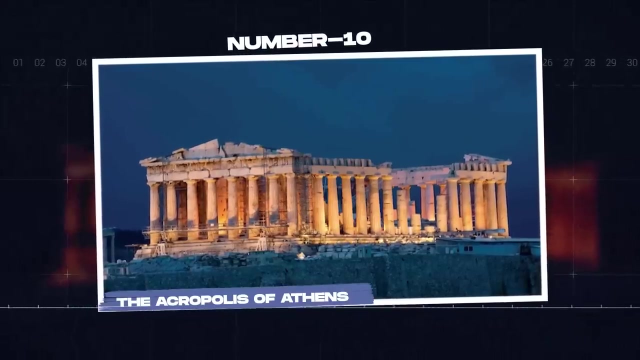 who was found with his weapons and armor intact. Was he killed in battle Or was his death the cause? The mystery only deepens when you consider that the warrior was buried alongside two women, one of whom may have been a shaman. 10. The Acropolis of Athens. 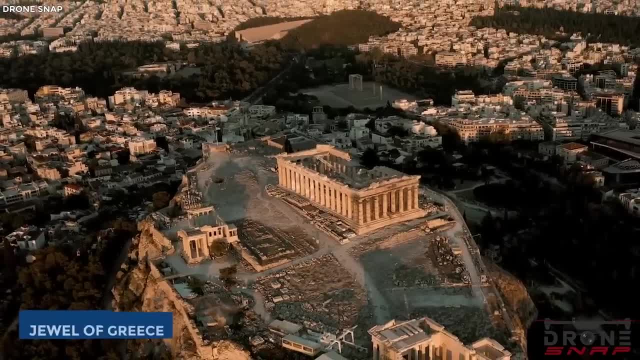 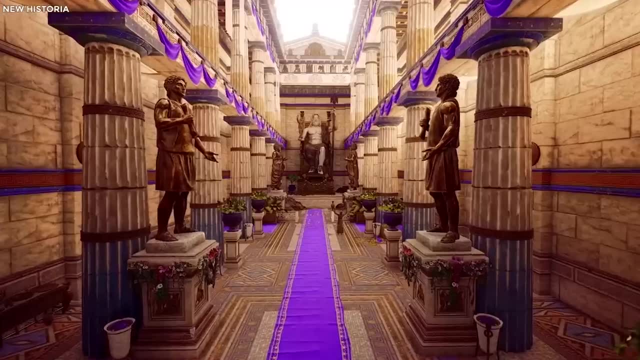 Let's move forward to the Acropolis of Athens, the jewel of Greece, the crown jewel of ruins, the place where people from all over the world gather to take selfies and feel cultured. The Acropolis has a long and storied history, dating back to the 5th century BC. It was built. 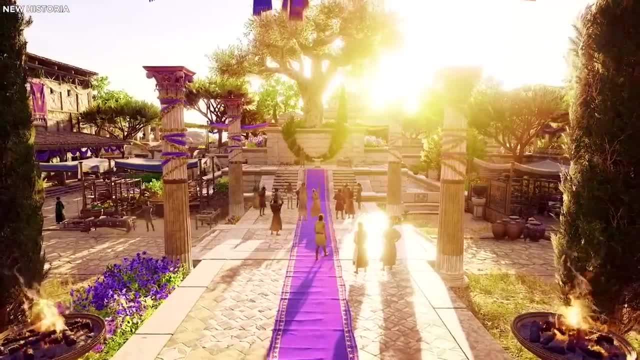 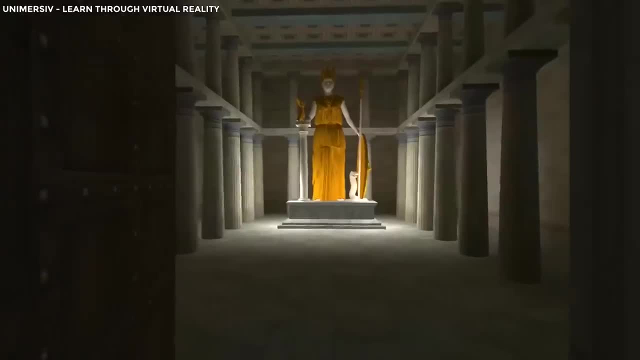 during the Golden Age of Athens, a time of great prosperity and cultural achievement. The Acropolis was the center of religious and cultural life in Athens, and it was home to several temples, including the famous Parthenon, One of the most striking features of the Acropolis. 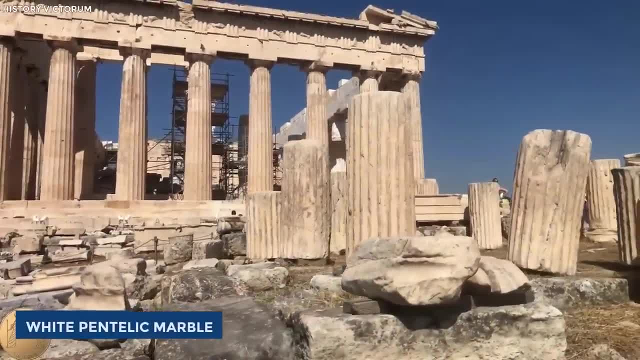 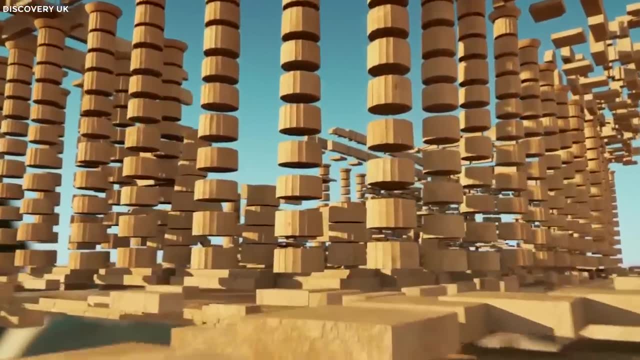 is its use of marble. The entire site is built from white pentelic marble, which was quarried just a few miles away from the Acropolis. This marble is known for its purity and fine grain, and it was highly prized by the ancient Greeks for its beauty and durability. 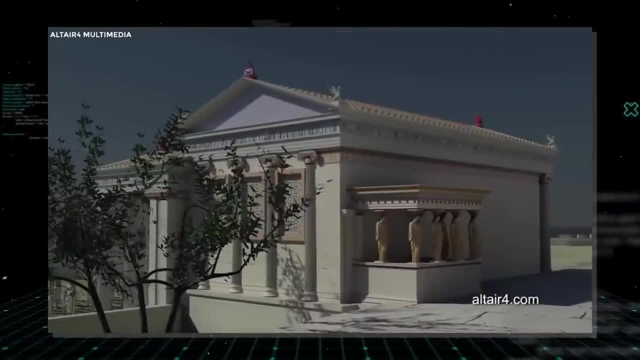 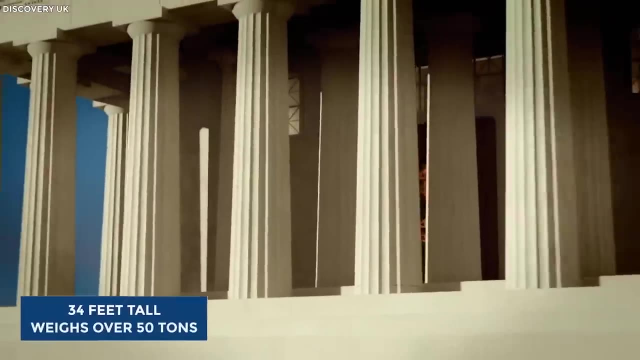 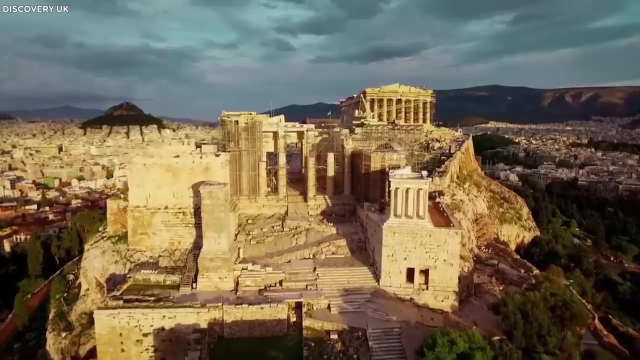 The most famous building on the Acropolis is the Parthenon, which is a masterpiece of symmetry and balance. The Parthenon is made up of 46 columns, each of which is 34 feet tall and weighs over 50 tons. The columns are perfectly spaced and angled, creating an optical illusion that makes 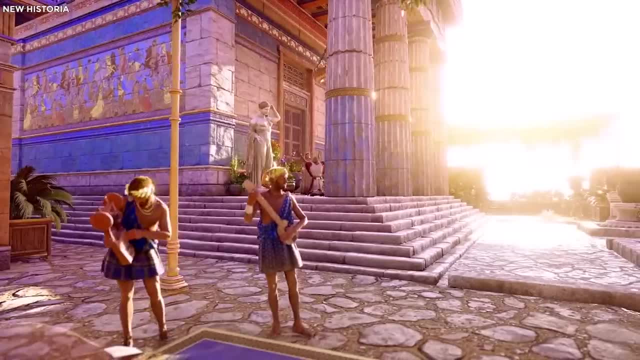 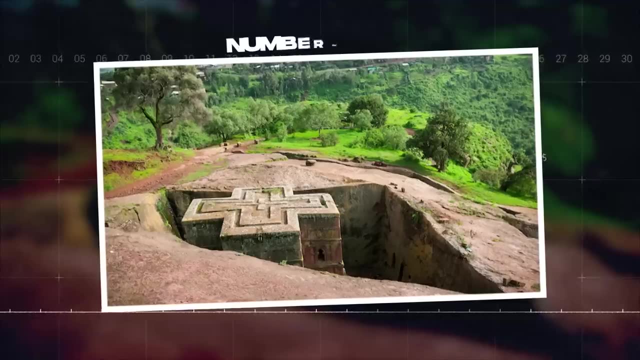 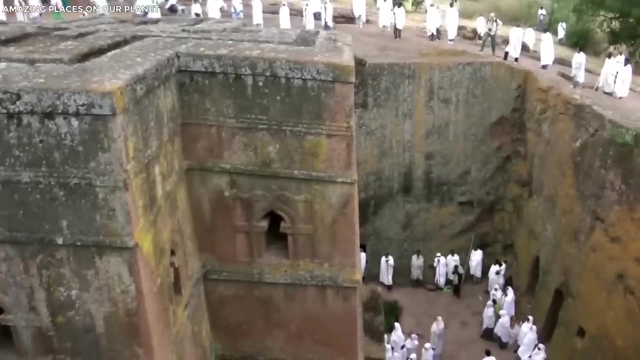 them appear perfectly straight from any angle. The Acropolis has also had a tumultuous history, but it still stands as a testament to the ingenuity and perseverance of the ancient Greeks. 9. Lalibela Churches. Moving on to Lalibela Churches, the place where history meets the undead, 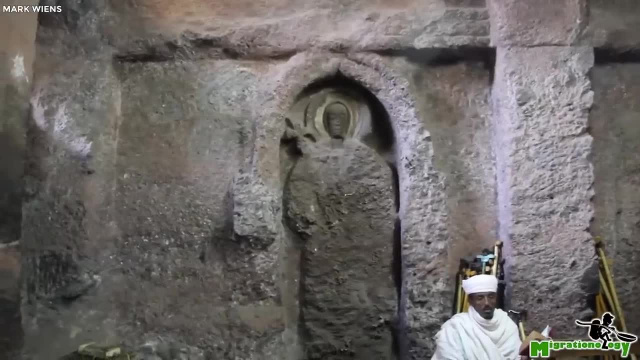 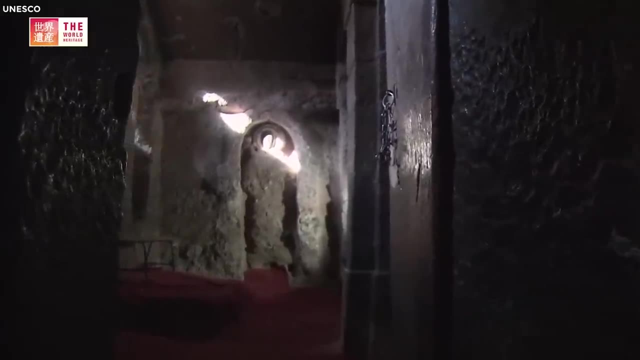 Yes, you heard that right. The mummies of Lalibela Churches are just as famous as their monolithic churches. But don't worry, these mummies won't give you nightmares, Or will they? Legend has it that these mummies are actually the remains of ancient kings who ruled Ethiopia. 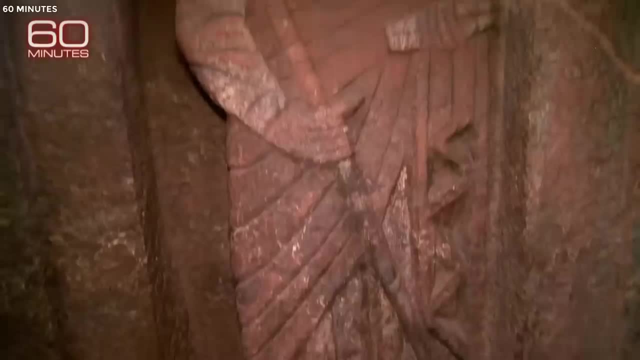 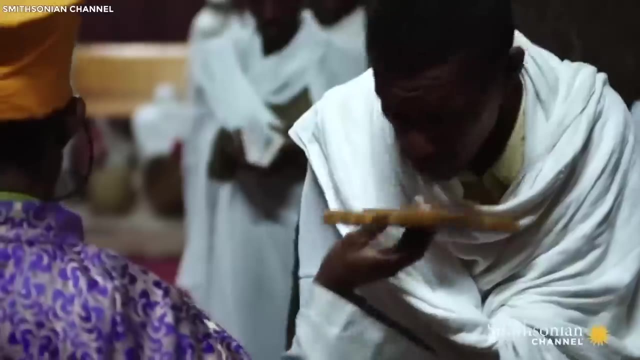 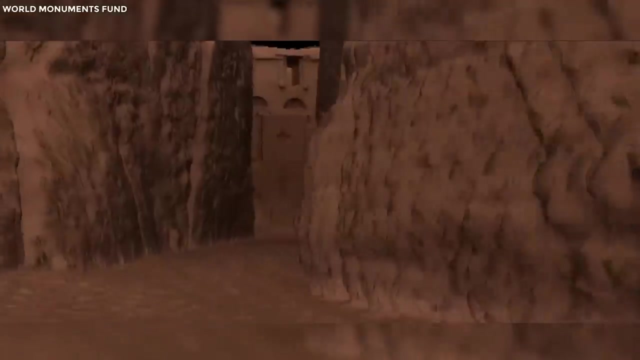 And let us tell you, these kings must have really loved their bling, because their mummified remains are adorned with gold crowns and jewelry. According to myths and mysteries, King Lalibela was visited by angels in his dreams and instructed to build these monolithic churches, And he really took that instruction to heart. 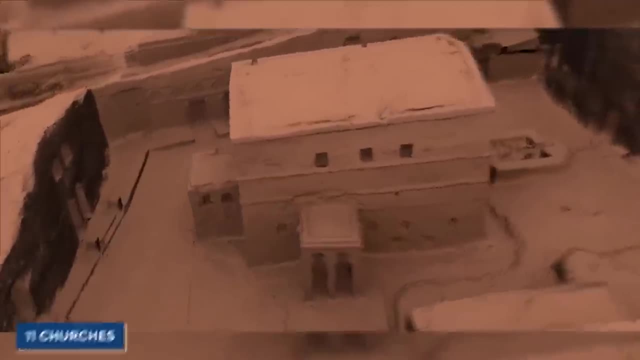 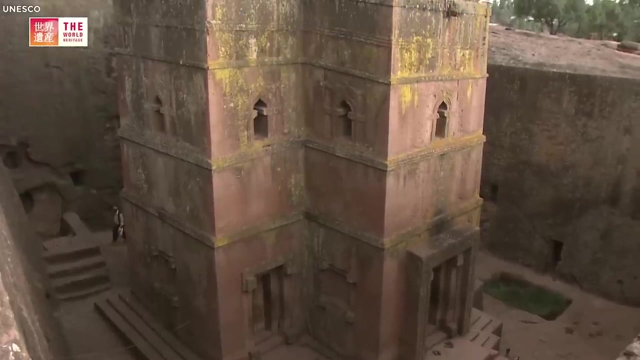 because he built not one, not two, but eleven churches. That's some serious commitment. Each one has its own distinct style and features intricate carvings and stunning artworks. The churches are also interconnected by a network of tunnels and walkways, making it easy for 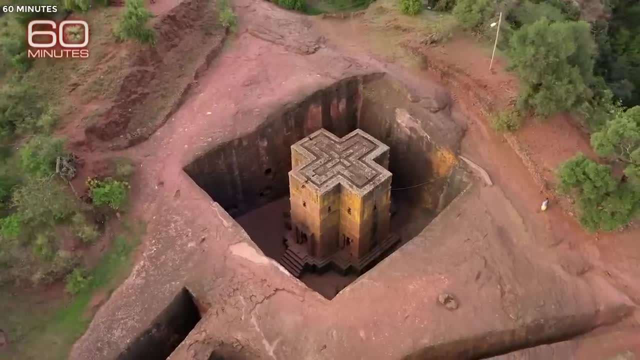 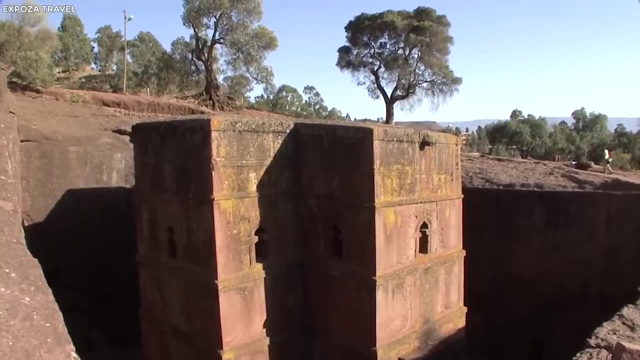 visitors to explore them all. And these churches aren't your run-of-the-mill buildings. They're carved out of solid rock. Who needs bricks and mortar when you can just carve your church out of a mountain? It's like the original man cave but for monks. But it's not just the impressive. 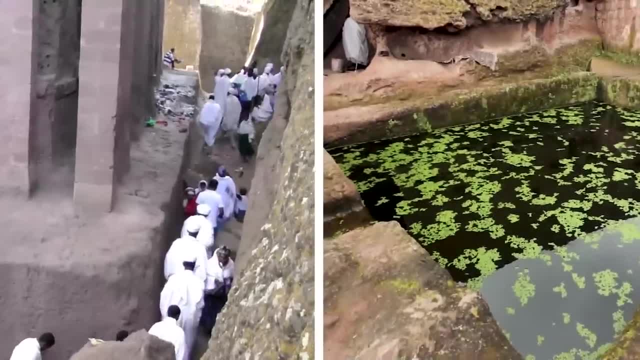 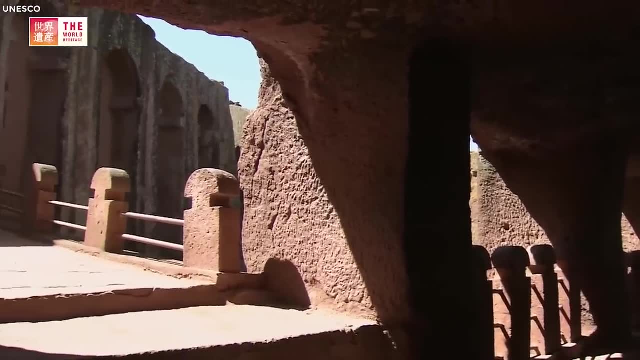 construction that makes these churches special. They also feature ceremonial passageways and an extensive drainage system. 10. Lalibela Churches. 8. Lalibela Churches. 10. Lalibela Churches. 12. Lalibela Churches. Calabela churches were not discovered in the traditional sense as they have been known and 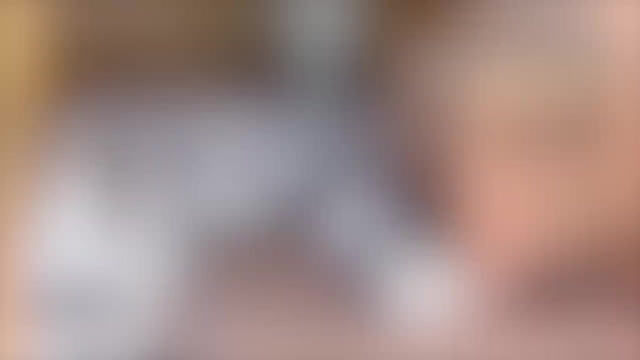 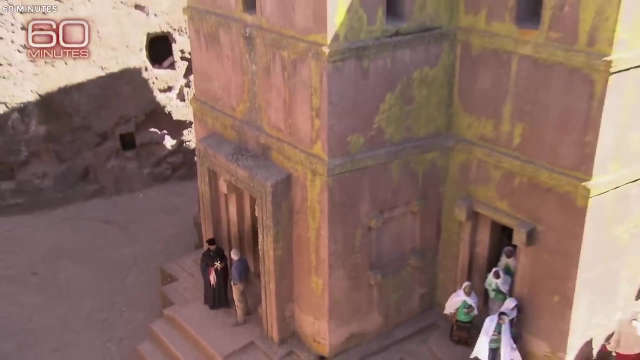 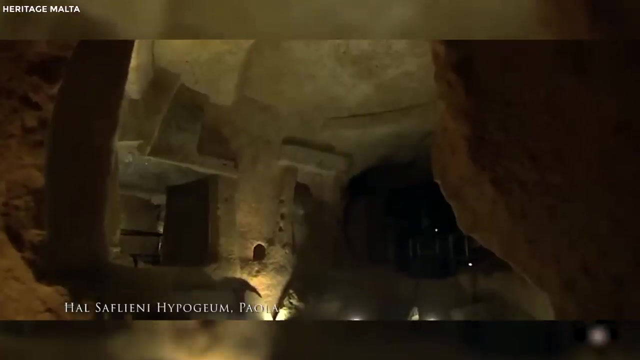 used for centuries by Ethiopian Orthodox Christians. However, the churches did gain international attention in the 20th century when they were explored and documented by scholars and archaeologists. 8. Hal Saflieni, Hippogym. Hold on to your hard hats, folks, because we're about to dig deep into the mysterious world of 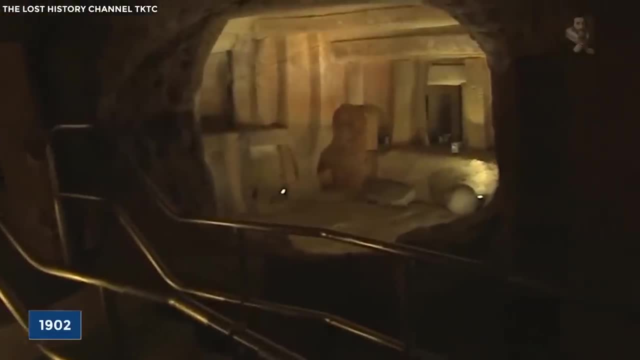 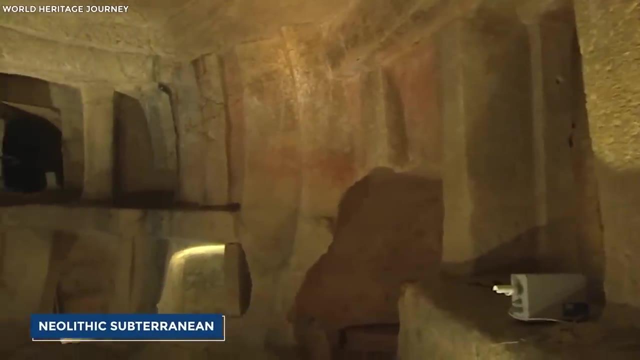 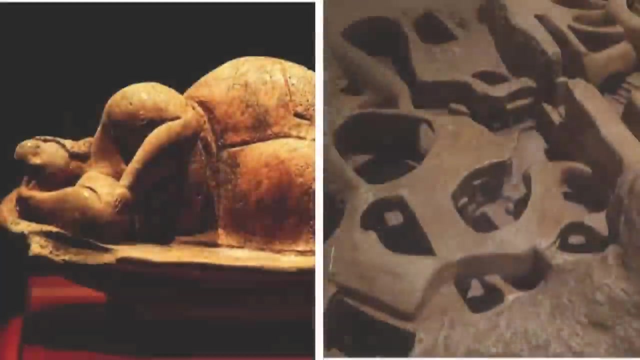 the Hal Saflieni Hippogym. It all started back in 1902, when some construction workers in Paola, Malta, accidentally discovered a Neolithic subterranean structure. while cutting cisterns Within the Hal Saflieni Hypogeum, there were discoveries of burial items- human remains. 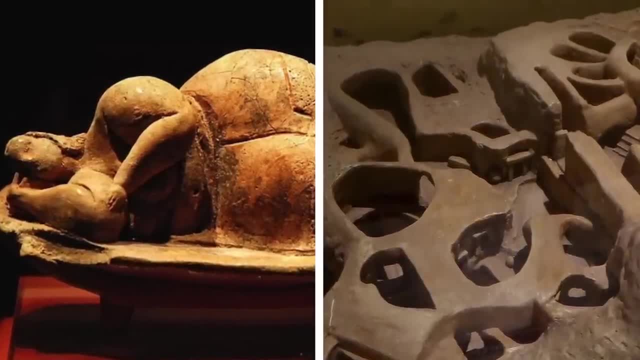 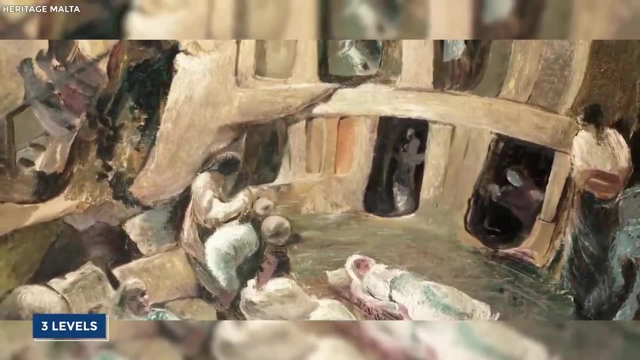 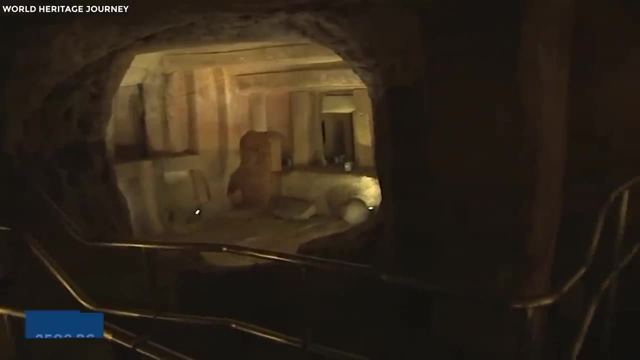 and a complex system of interconnected chambers on multiple levels Chilling right. The Hypogeum consists of three levels, each dug into the soft limestone bedrock. The lowest level is the oldest, dating back to around 3600 BC, while the uppermost level was built around 2500 BC. 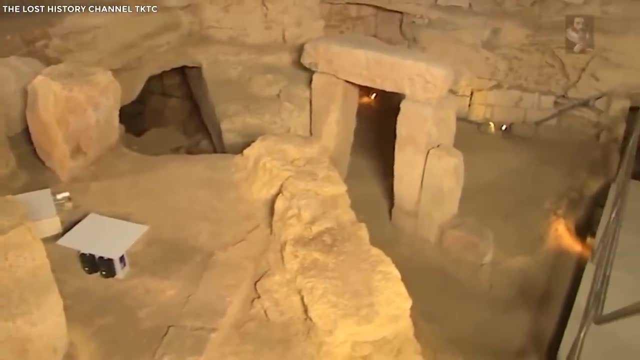 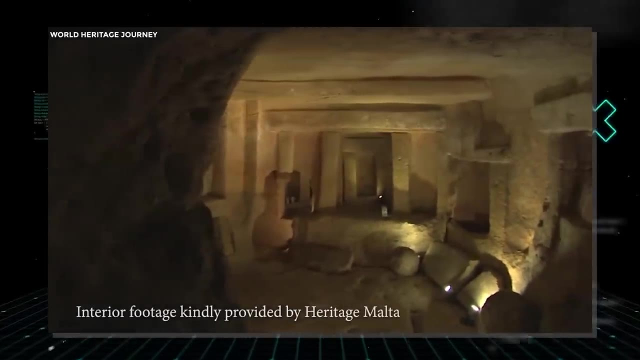 The entire complex was used for ritual and burial purposes, and it is believed that thousands of people were buried there over the course of several centuries. The chambers themselves are stunning, with smooth walls that curve and undulate like waves. The acoustics in the 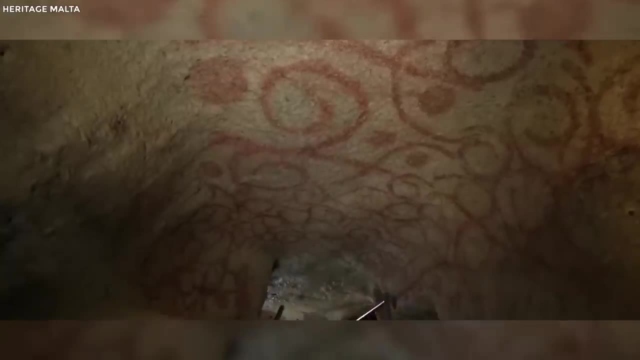 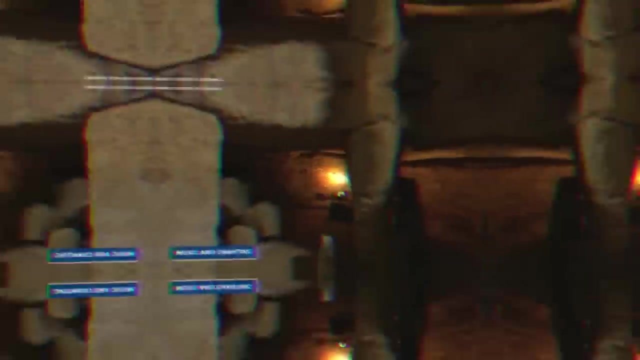 Hypogeum are also remarkable. It's been said that the space has a perfect acoustic resonance, which has led some to speculate that it was used for music and chanting during rituals. But the Hypogeum is not without its mysteries. One of the most puzzling is the fact that there 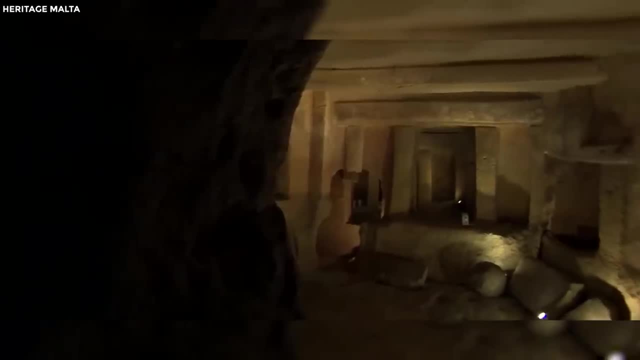 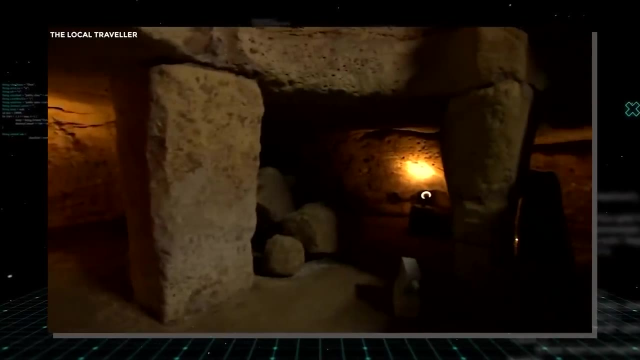 are no windows or chimneys in the complex, and yet the air inside remains fresh and breathable. Some have speculated that the complex was ventilated through a series of shafts that have yet to be discovered. So if you're feeling brave enough, grab a flashlight and some sturdy. 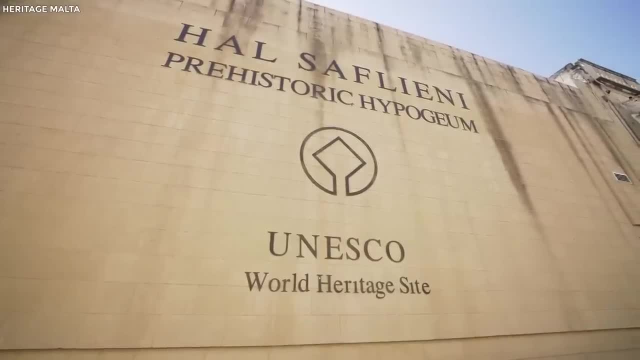 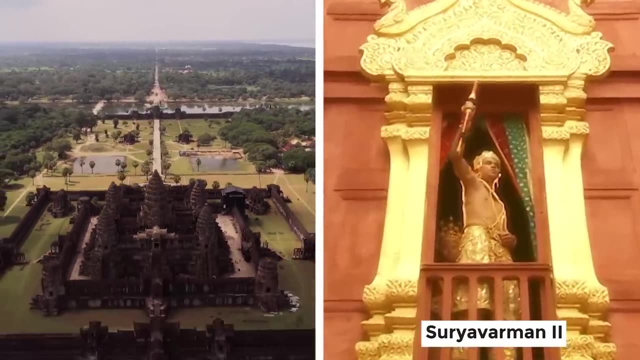 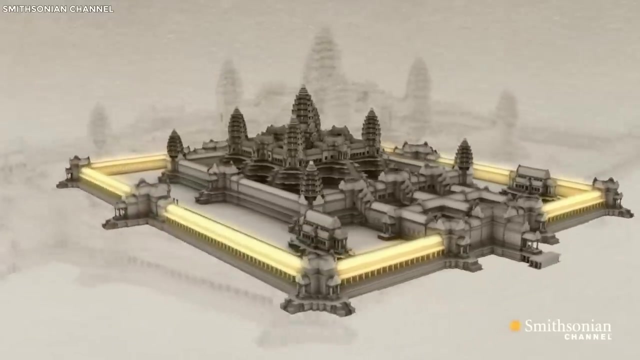 shoes and head down to the Hal Saflieni Hypogeum. 7. Angkor Wat. Angkor Wat built in the 12th century under King Suryavarman II's rule as a temple devoted to the Hindu deity Vishnu. It is like the Meryl Streep of religious monuments. 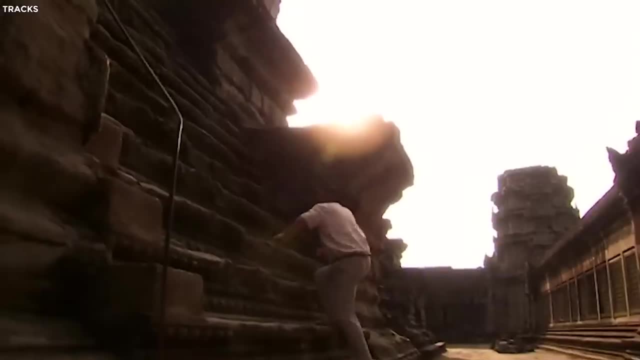 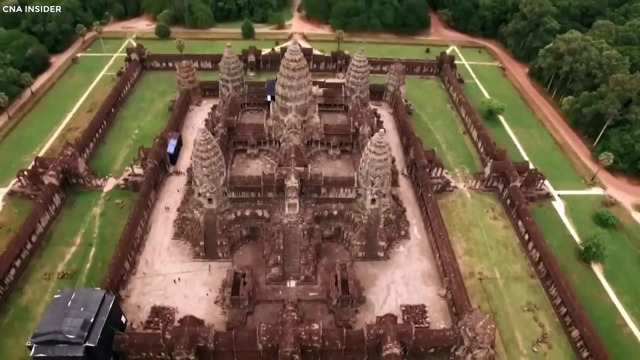 everyone's talking about it and it's won all the awards. And you know who we have to thank for this: A French naturalist. But with time, the temple was then adapted by Buddhists and evolved into the structure we know today. This transition was reflected in the temple's 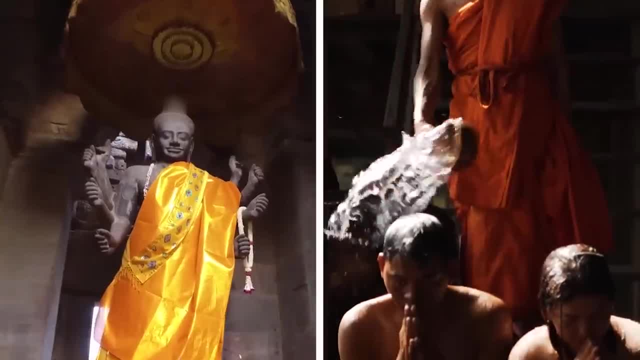 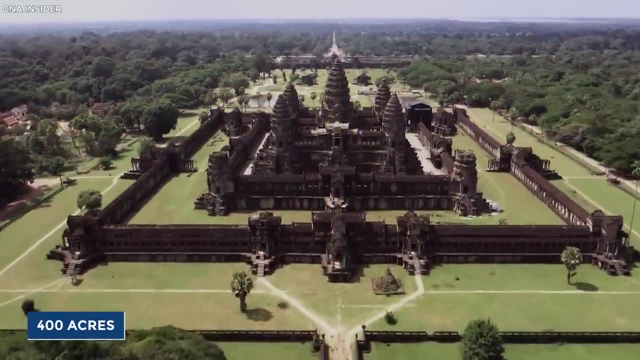 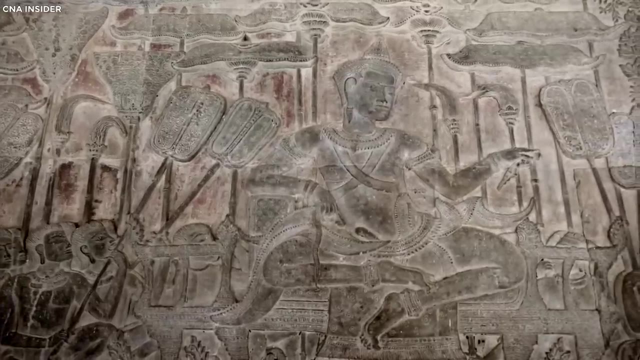 religious beliefs of the Khmer people, who were a melting pot of Hindu and Buddhist cultures. The temple complex itself is massive, covering an area of over 400 acres. It consists of three levels, each representing a different level of heaven in Buddhist cosmology. 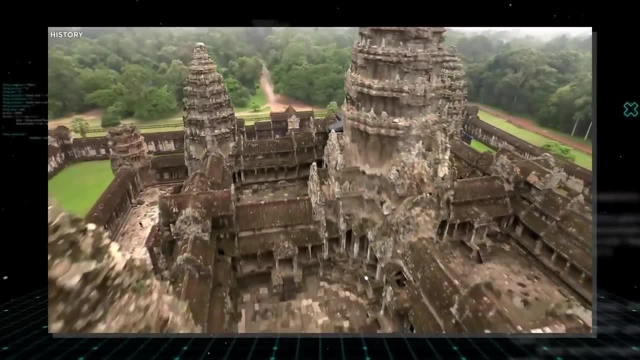 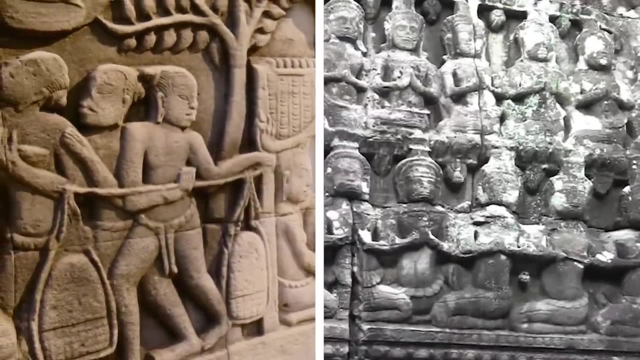 One of the most impressive features of Angkor Wat is its intricate carvings. The temple is covered in thousands of stone carvings depicting everything from Hindu and Buddhist mythology to scenes from ancient history. The temple is also a place where you can find a lot of 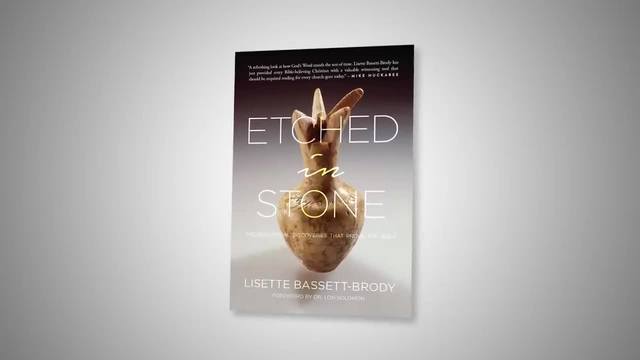 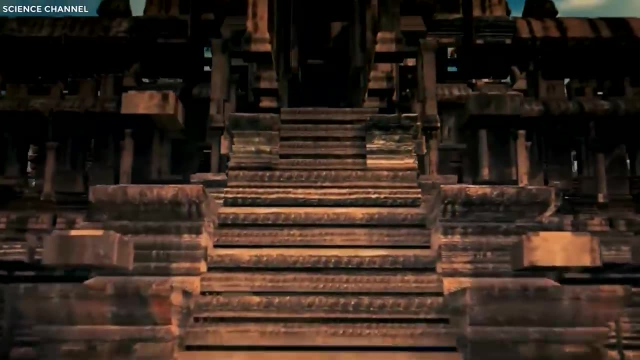 everyday life in ancient Cambodia. It's like a giant history book etched in stone, telling the story of a civilization that existed over 800 years ago. It's no surprise that this awe-inspiring wonder of the world is a source of pride for the Cambodian. 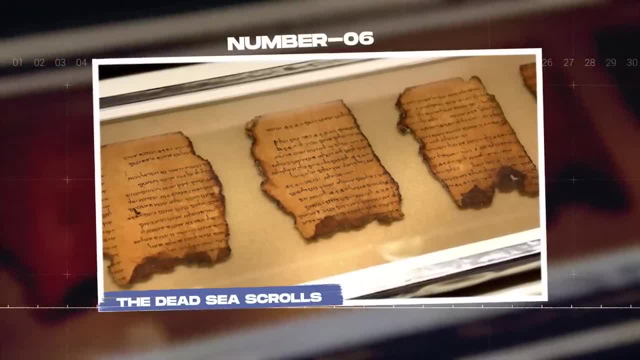 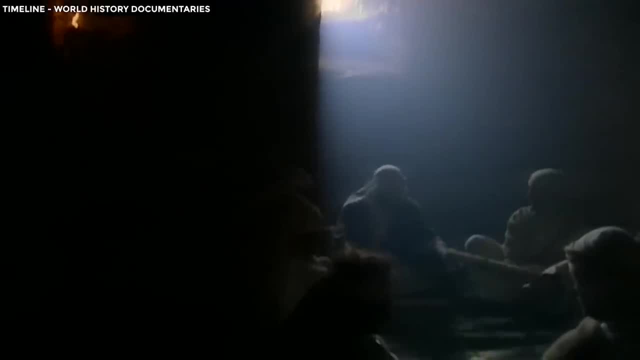 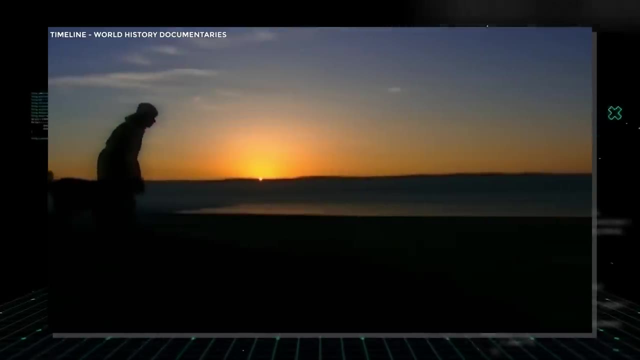 people. 6. The Dead Sea Scrolls. The Dead Sea Scrolls: Just the name alone conjures up images of mystery and intrigue, of long-lost secrets hidden away in the depths of the desert. In 1947, a Bedouin shepherd stumbled upon one of 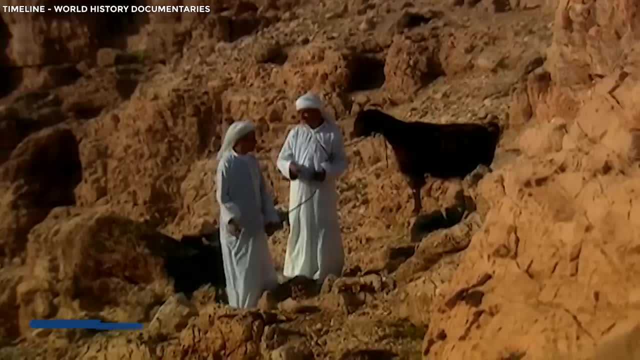 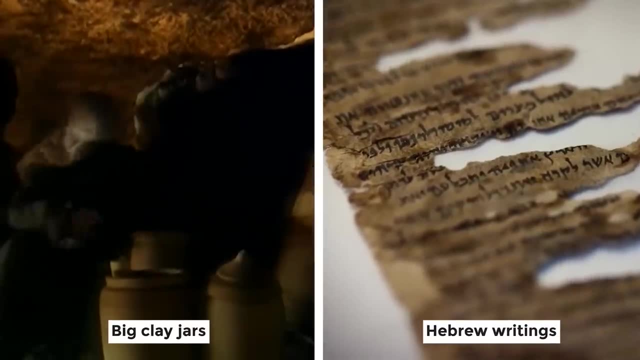 the greatest archaeological finds in history, while tending to his flock in the Judean desert. Who knew that goats could be such great explorers? The scrolls were found in big clay jars and had Hebrew writings that were more than 1,000 years older than any existing Bible texts. 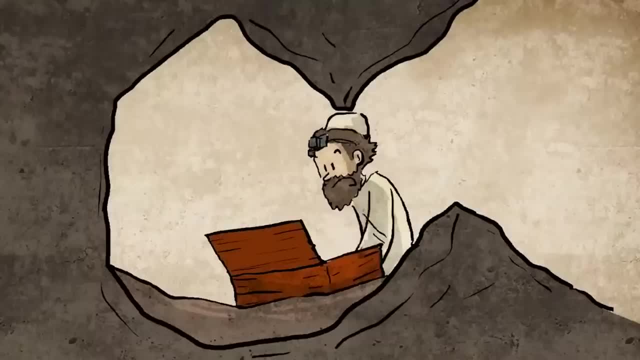 The scrolls were written in Hebrew, Aramaic and Greek and date back to the Second Temple period of 538 AD. The scrolls were written in Hebrew, Aramaic and Greek and date back to the Second Temple period of 538 AD. 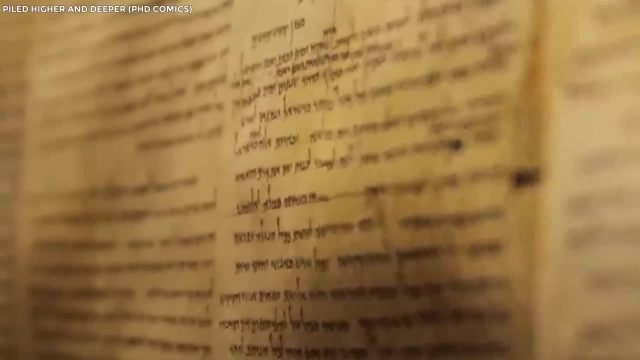 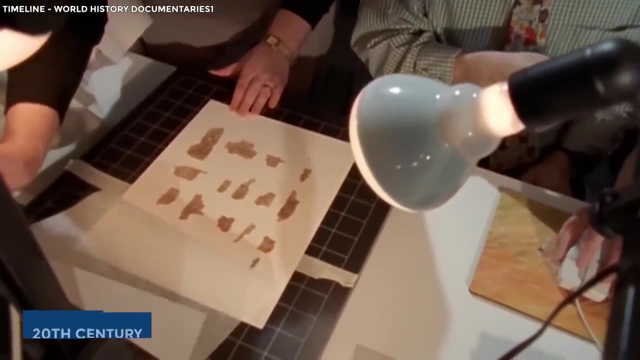 The scrolls were written in Hebrew, Aramaic and Greek and date back to the Second Temple period of 538 AD. They include religious texts, hymns, prayers and historical accounts, and are considered by scholars to be among the most significant discoveries of the 20th century. 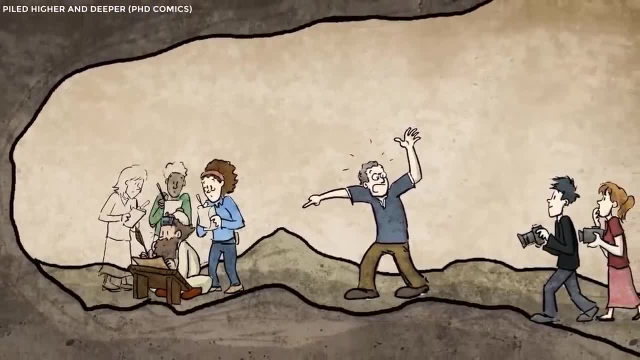 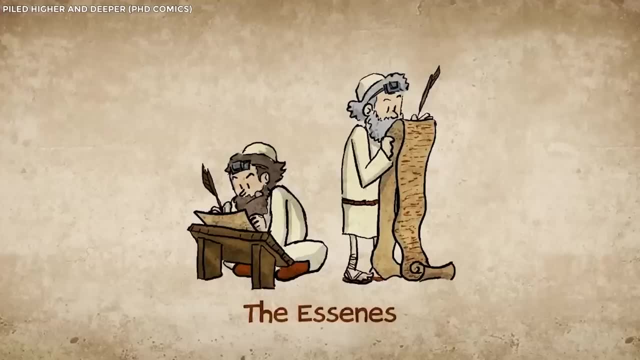 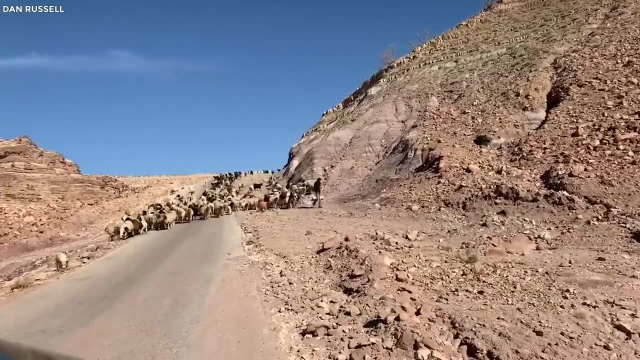 But the Dead Sea Scrolls are more than just ancient documents. They have revolutionized our understanding of the development of Judaism and Christianity, shedding new light on the religious beliefs and practices of the time. So let's raise a glass of holy water to the Bedouin shepherd. 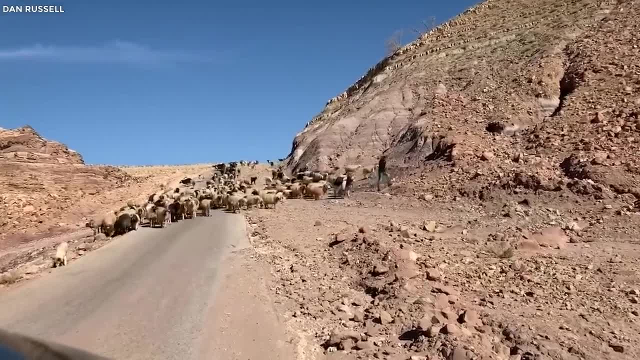 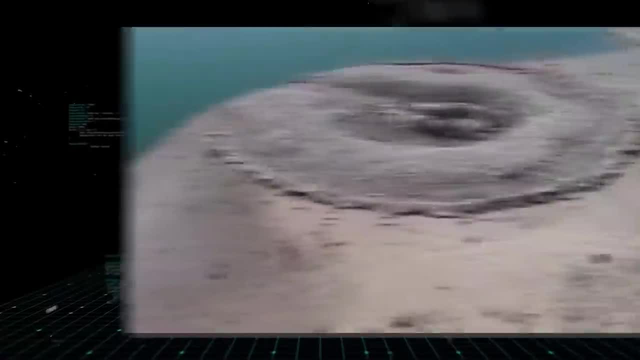 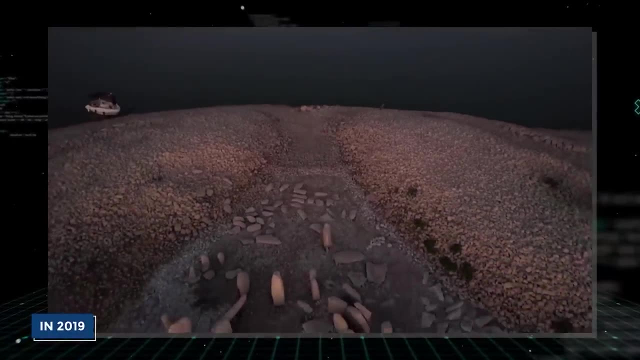 who stumbled upon this incredible find. 5. Spanish Stonehenge. Are you ready for a tale of adventure and discovery? Well, get ready to be amazed, because a drought in Spain's Extremadura region in 2019 led to the discovery of a fascinating ancient site Known as the Dolmen de Guadalperal, or the Spanish 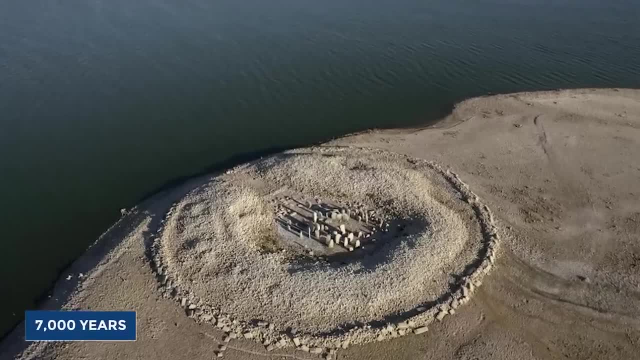 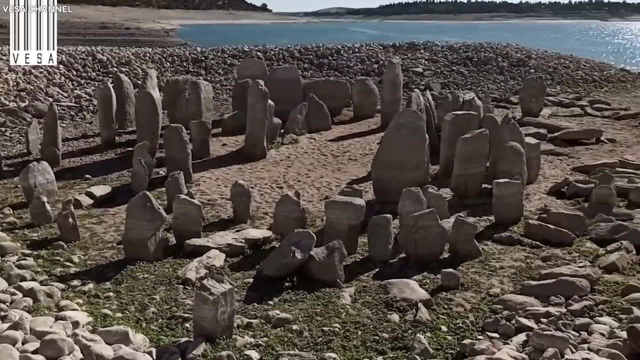 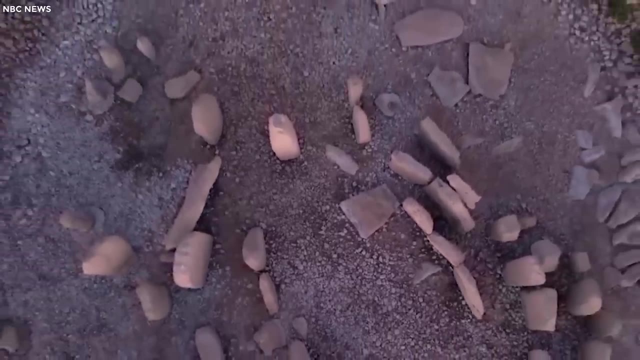 Stonehenge. this submerged wonder dates back 7,000 years and contains 100 monolithic stones, some towering at a height of 6 feet. The building showcases an insane amount of precision and even reflects. whoever built this site had a deep understanding of mathematics and geometry. 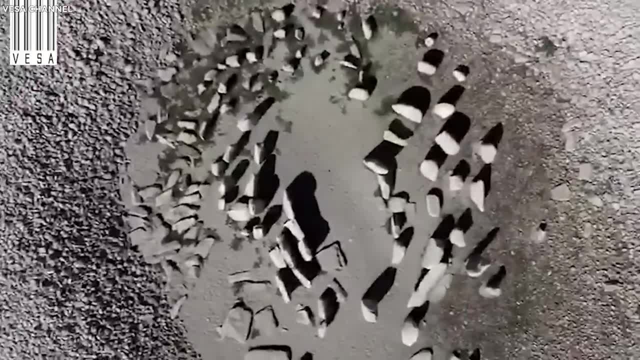 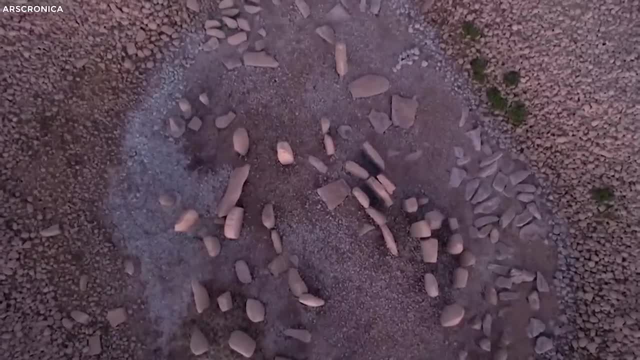 Why you ask. It's because the stones are so precisely arranged that they create a series of geometric shapes, including triangles and rectangles, And the monolithic stones are arranged in a circular pattern, with some of them forming an archway that would make even 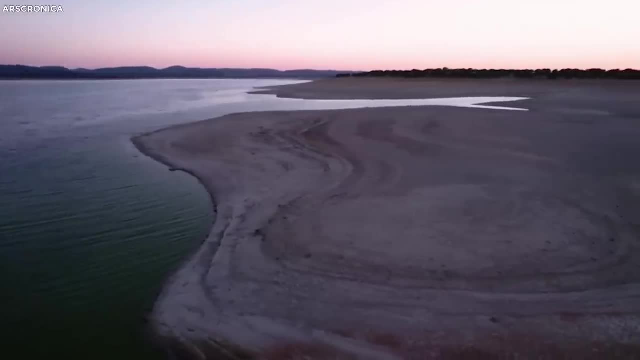 the most seasoned architect, jealous. It's believed that these stones were used to build a tower, a temple or a church. These stones were used in some sort of ritualistic or religious practice, but the exact purpose is still shrouded in mystery. 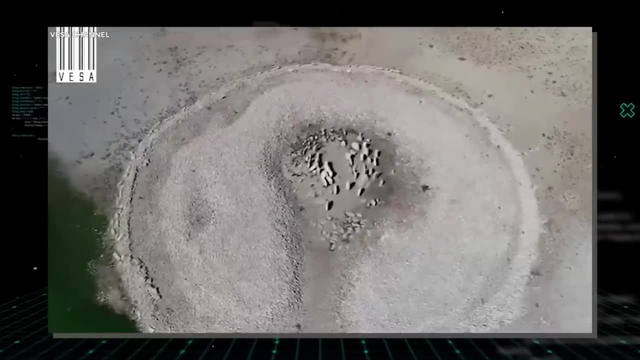 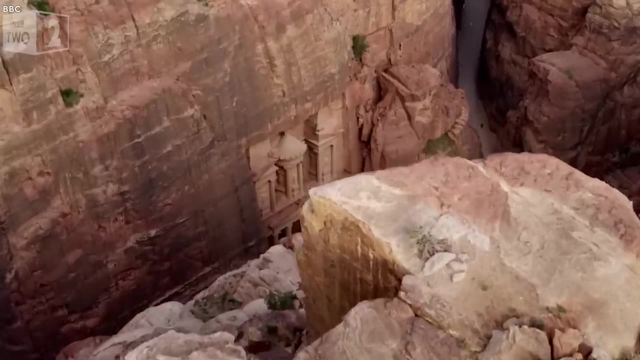 It may not be as famous as its British counterpart, but it's just as amazing and mysterious. 4. Petra. Now, our next spot is the Lost of Petra, which played the greatest game of hide-and-seek with the world for centuries. This ancient city, 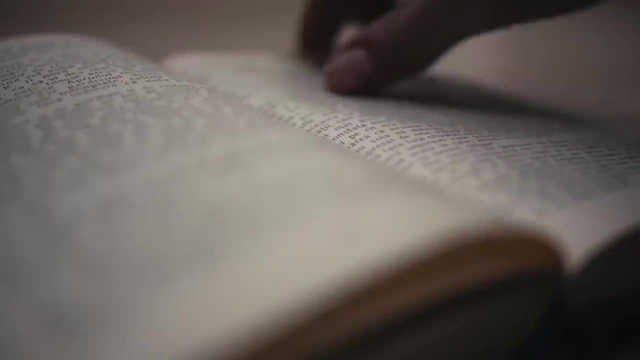 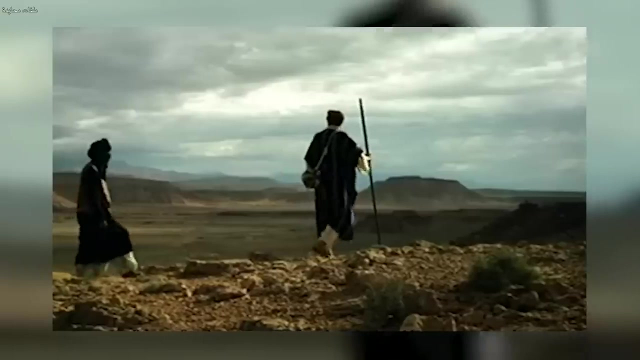 had been referenced in historical documents, but nobody had been able to find it. But then, in 1812, along came Swiss explorer Jean-Louis Burckhardt, who was pretty much like Indiana Jones on steroids: He was determined to find Petra, no matter what, And after months of searching. 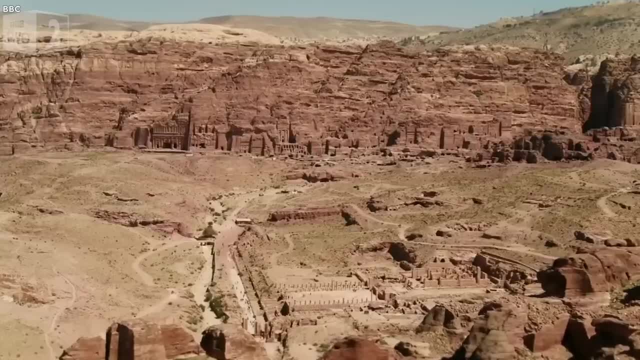 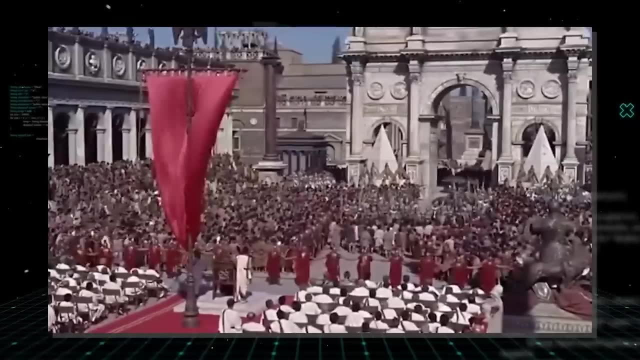 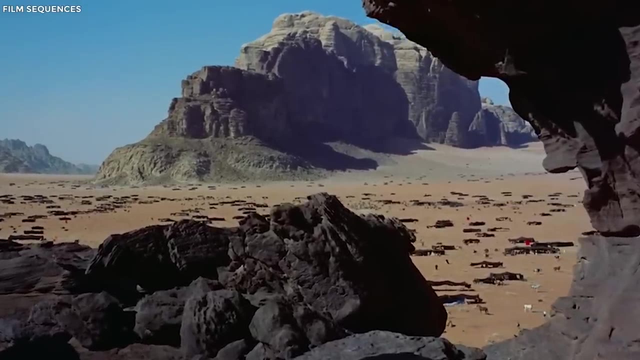 he finally stumbled upon the entrance to the city, And what a city it was. Petra was first inhabited in 7000 BC and it's believed that the Nabataeans, a nomadic Arab people, settled there around 300 BC. The city was a major trading hub focused on wealth and commerce. 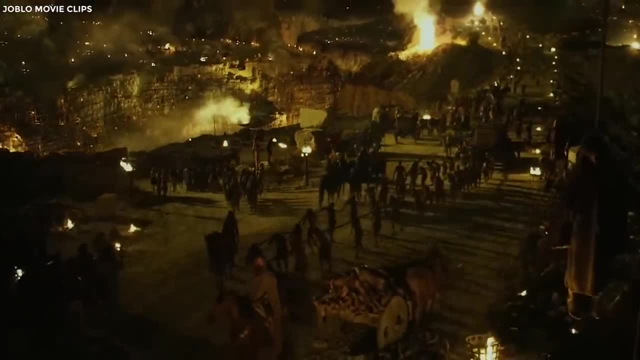 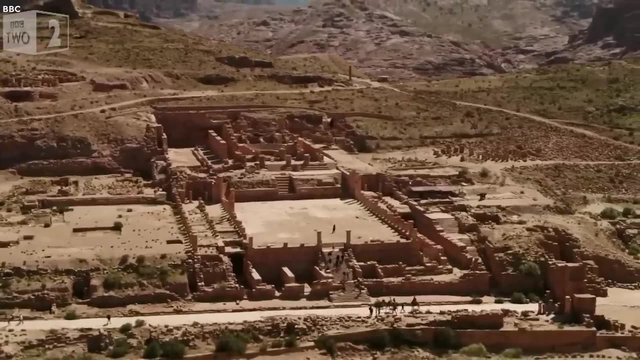 and it's easy to see why The city is filled with stunning architecture and intricate carvings that would have made it a prime destination for traders and merchants. Walking through the city, you'll see the remnants of a once-thriving metropolis, complete with a theater, temples, 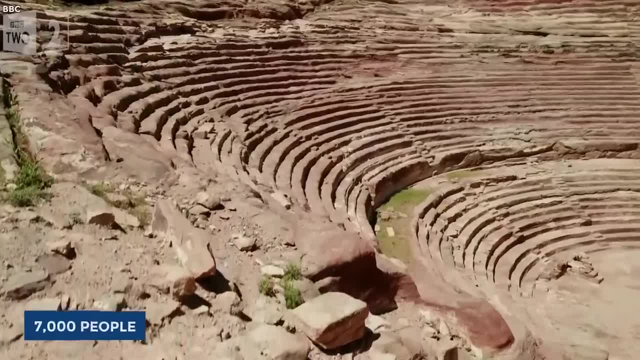 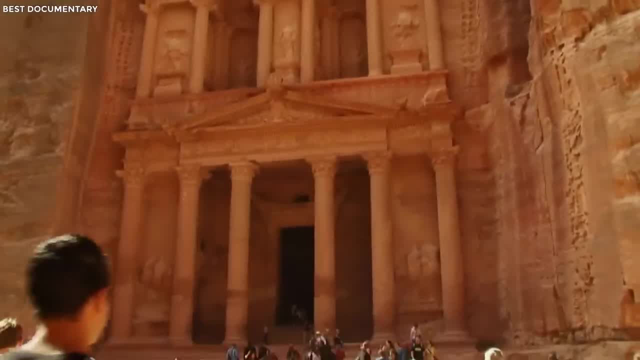 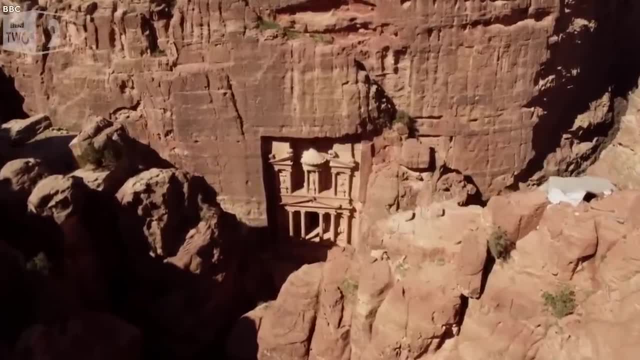 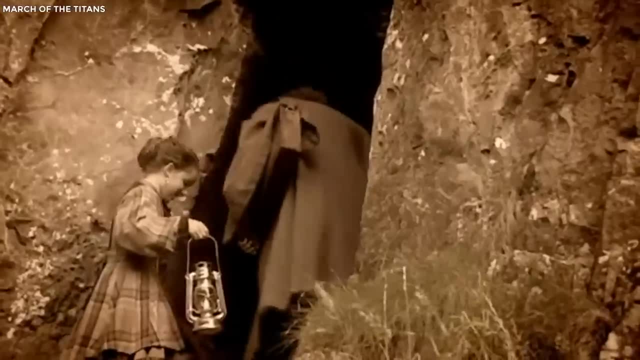 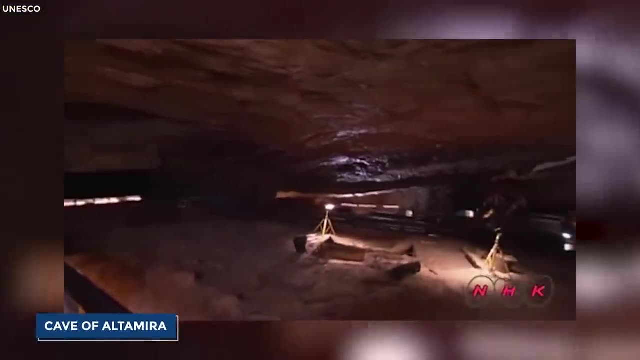 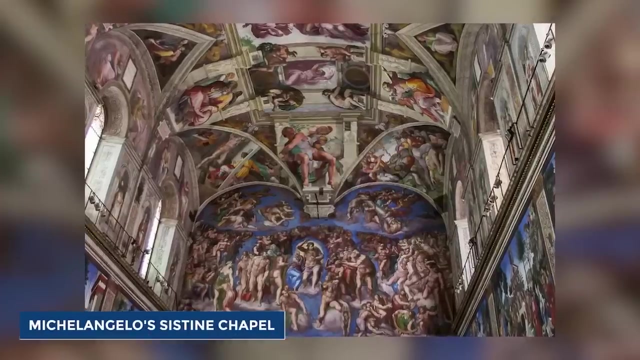 3. Cave of Altamira. As we delve into the depths of history, we come across a cave that is not just any cave: It's the Cave of Altamira. Imagine stumbling upon a cave with stunningly preserved paleolithic paintings that make Michelangelo's Sistine Chapel look like a kindergarten drawing. 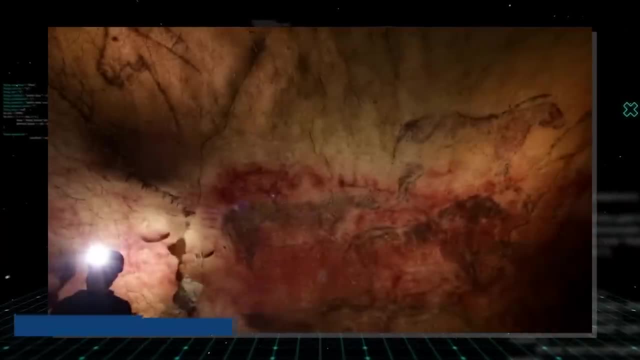 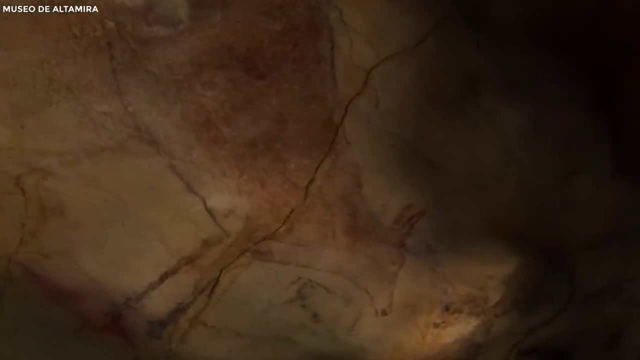 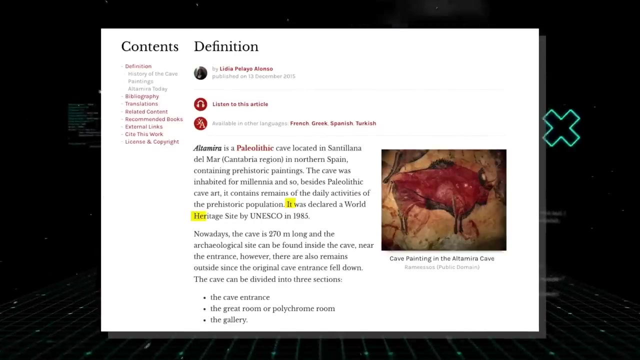 The cave is located in northern Spain and contains over 270 charcoal and polychrome paintings, including depictions of bison, horses and human hands. These drawings date back to the Upper Paleolithic period, making them approximately 35,000 years old. In 1985, UNESCO declared the cave a World Heritage. 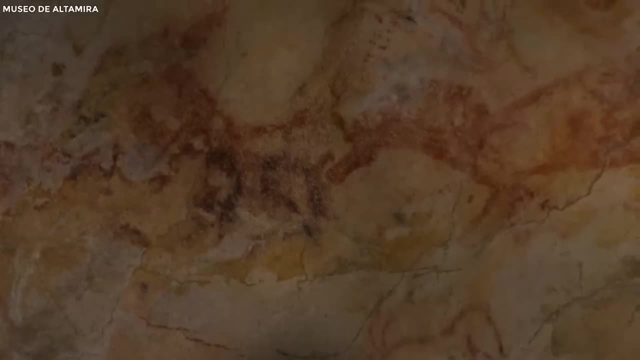 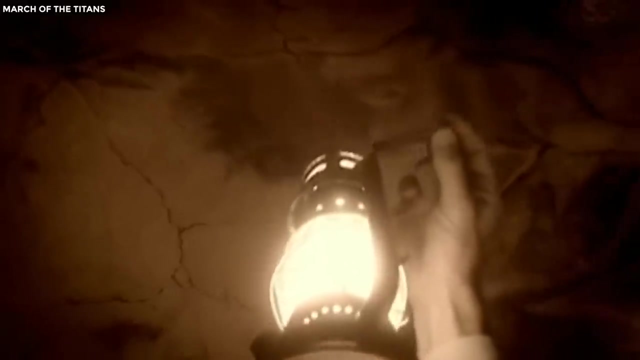 Site, recognizing its significance as an invaluable record of the prehistoric human way of life. The artwork found in the Cave of Altamira is said to be one of the most important discoveries in the history of prehistoric art. It's like the Mona Lisa of the cave world. Who knows what other. 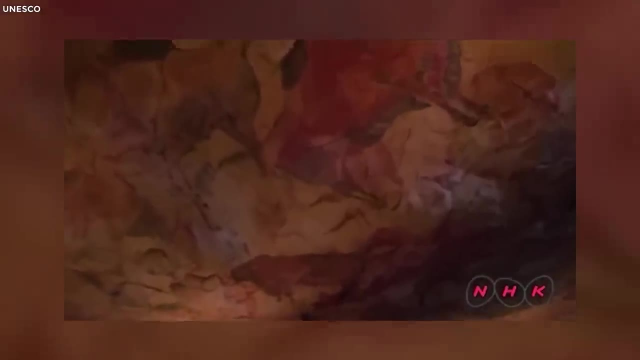 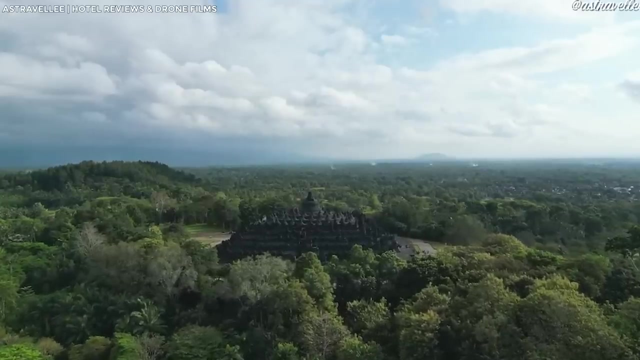 secrets this cave holds. Maybe there's a hidden stash of ancient paintbrushes somewhere in there. 2. Borobudur. Borobudur is one of the most stunning and biggest Buddhist temples, leaving the visitors to be left baffled by its structure. 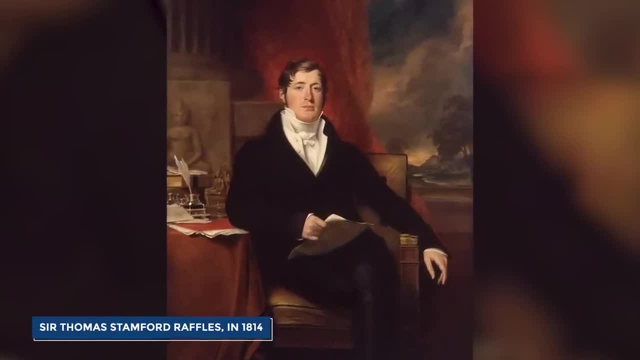 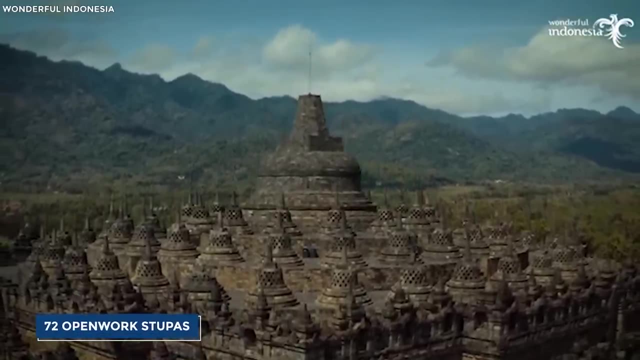 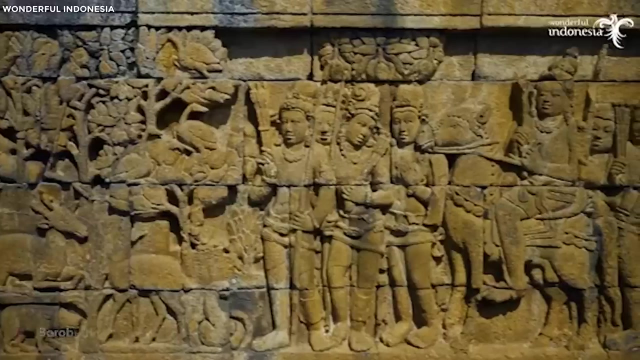 ever since it was discovered by Sir Thomas Stamford Raffles in 1814.. Built in the 9th century, the structure is a marvel, With 72 open-work stupas and stunning architecture which blends Indonesian and Indian cultures. the temple transports you back in time to a world where religion and spirituality 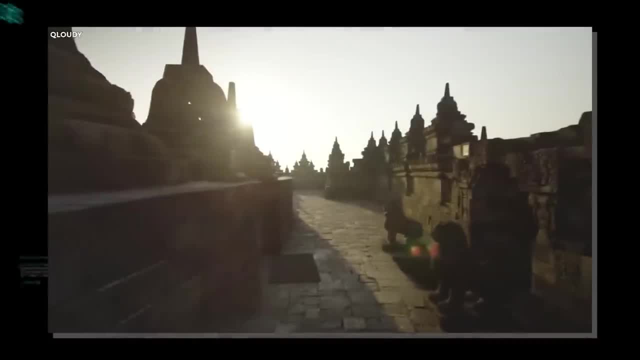 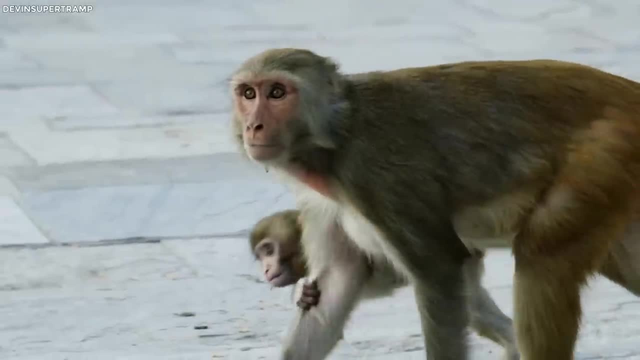 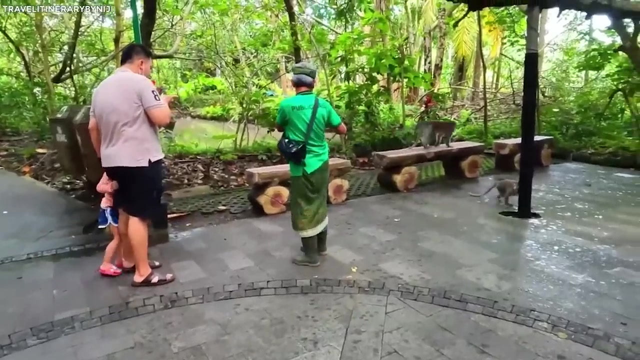 were at the forefront of everyday life. But isn't your regular temple with fancy designs also a place of pilgrimage for Buddhists from all over the world? And let's not forget about the monkeys. These playful creatures still roam the grounds of Borobudur, providing entertainment for visitors and reminding us of the temple's. 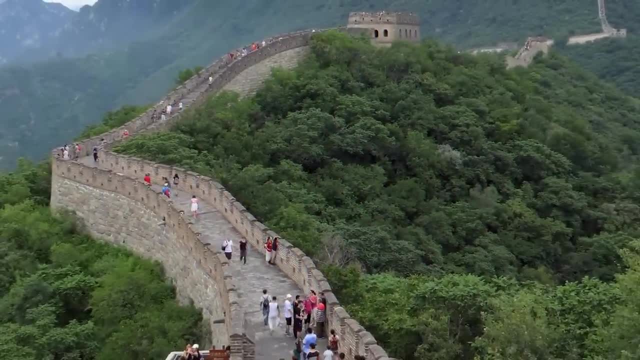 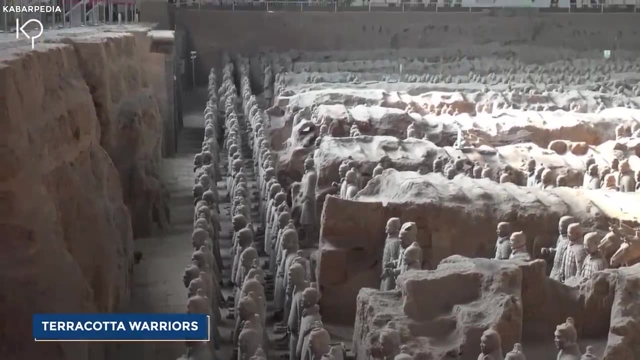 playful past. Prepare to be amazed, for today we're taking a trip to ancient China to witness one of the most astonishing discoveries of our time: the terracotta warriors. So picture this: it's 210 BC and Emperor Qin Shi Huang has just died. 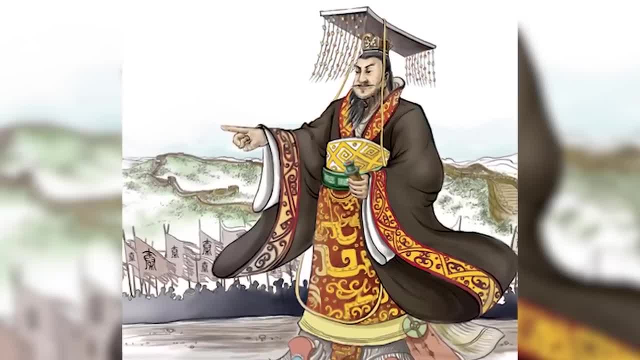 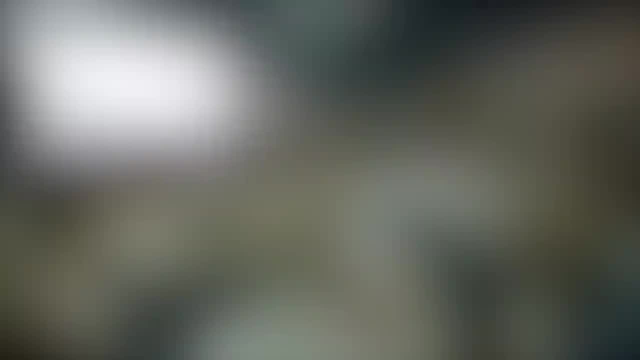 But this isn't just any ordinary death. Oh no, this is the death of a man who's determined to take his army with him to the afterlife. And what's the best way to do that, you ask? Well, obviously it's by building an army. 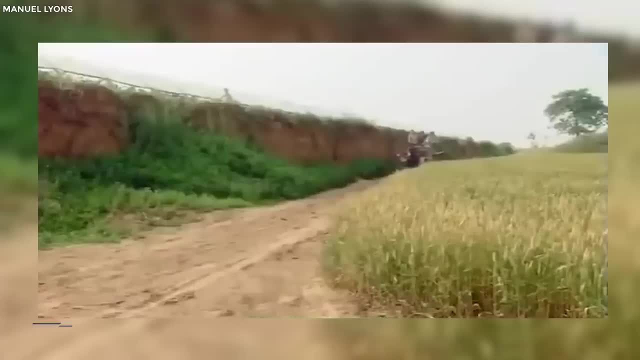 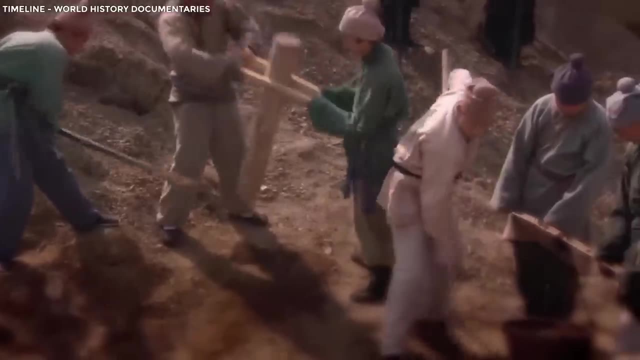 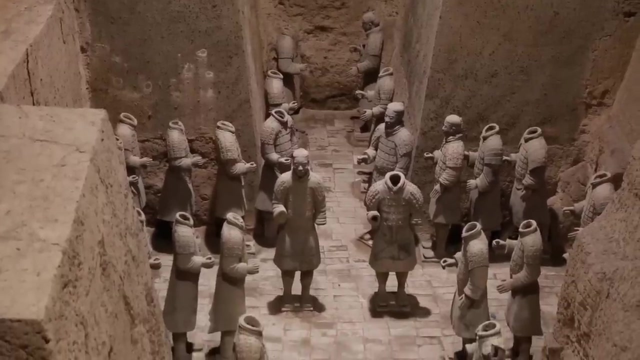 You can build an army of 8,000 life-size clay soldiers. Fast forward to 1974, and some farmers are just minding their own business tilling their fields. when they stumble upon the motherlode, That's right, they find the terracotta warriors. The terracotta warriors aren't just any old army. 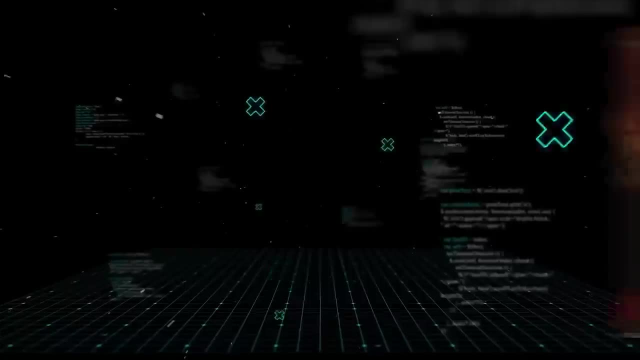 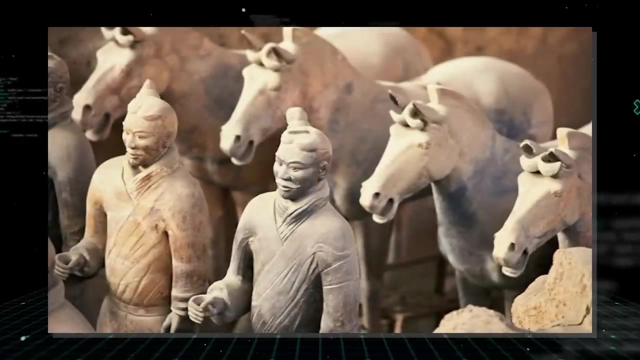 Oh no, they're a replica of the city of Xi'an. That's right. Emperor Qin Shi Huang built his own mini-city underground, complete with clay soldiers, horses and even chairs. But wait, there's more. Rumors have been swirling for years that there's even more to this tomb than